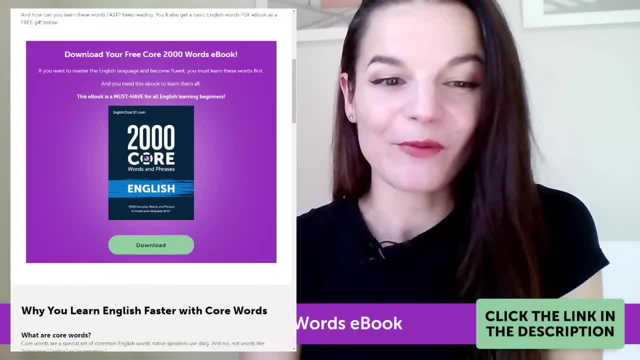 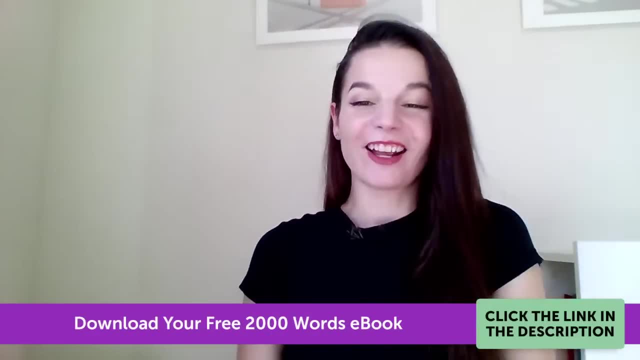 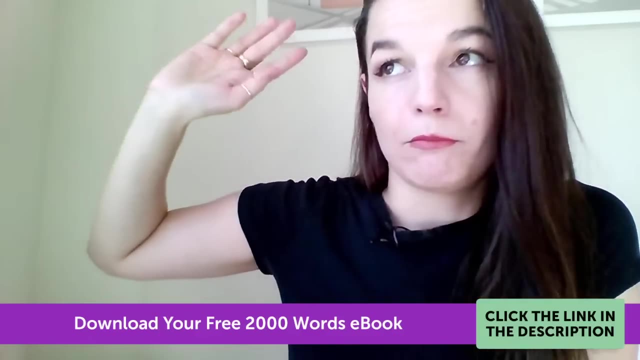 right. So this is a great tool to use For your vocabulary study. So go download that, Okay. Announcement number two: If you have questions for me that are different from today's lesson topic, send them not in the live stream chat, not an Instagram DM, not Facebook comments. I don't know, There are too many comments. 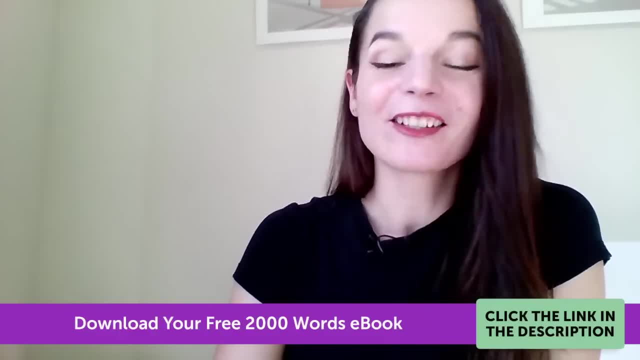 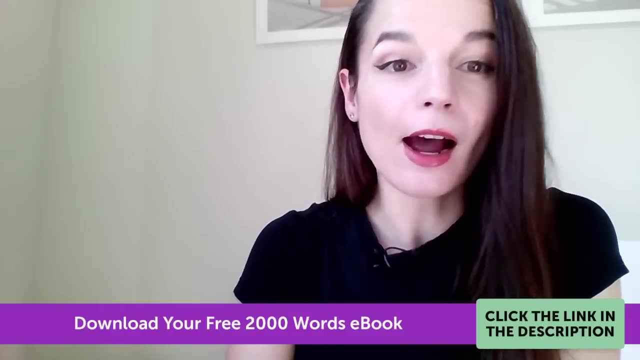 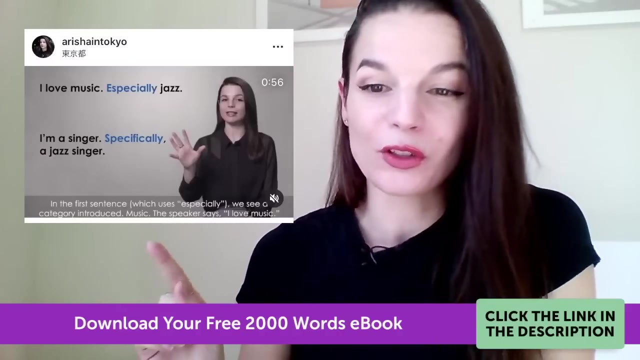 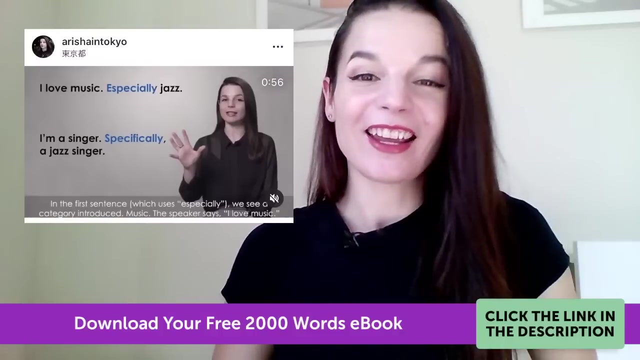 on all of our platforms. So please send me your questions to the official ask Alicia question submission page. Well, maybe choose your question to include in our weekly video. So this is a very, very old screenshot, but I choose your actual questions and I answer them, I hope and I include them. 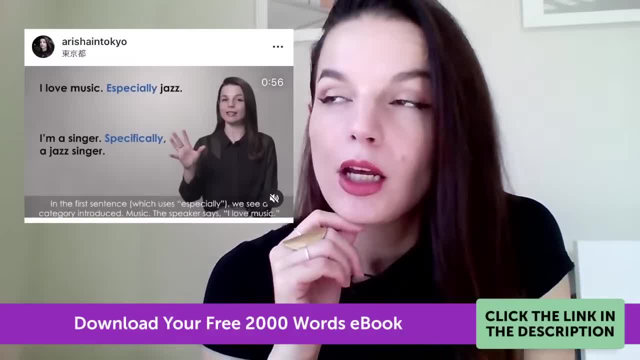 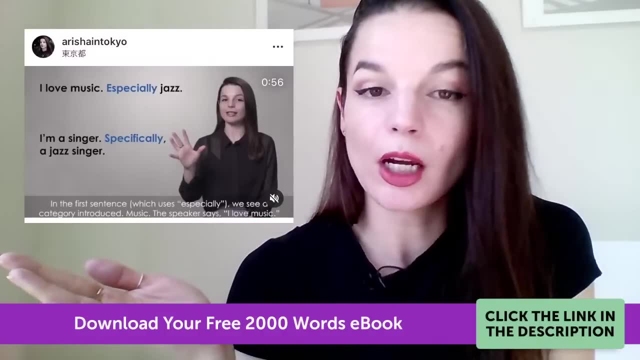 in these videos each week. So if you have a question, if you're watching a movie or you see something in a news article that's confusing, whatever send it to me. We can talk about it, but make sure you search the channel first, because maybe I've already answered. 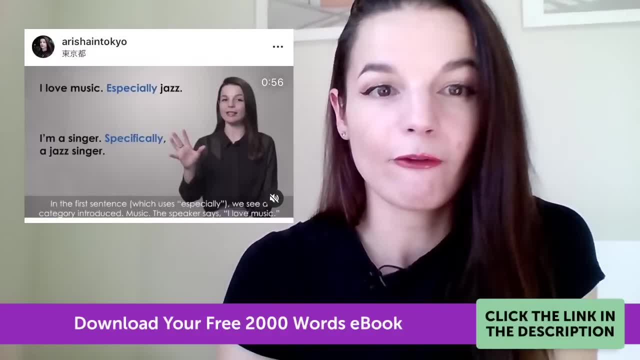 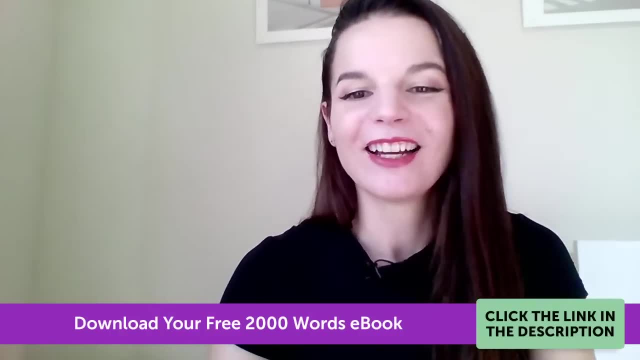 your question, Like if it's a preposition question. I have like 50 videos about that, So do yourself a favor and see if I answered your question already. Okay, That's all for my announcements. I think everything is rolling, Okay. Yeah, Team, All right. YouTube. What's up? YouTube? 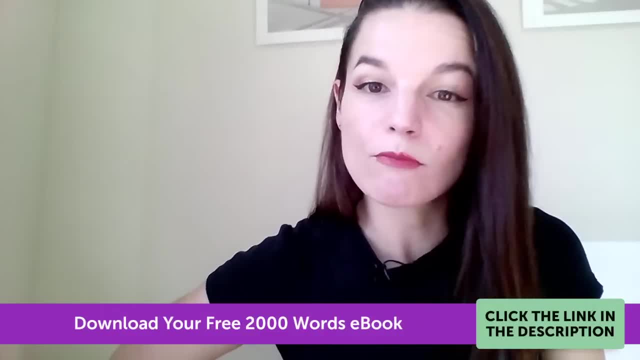 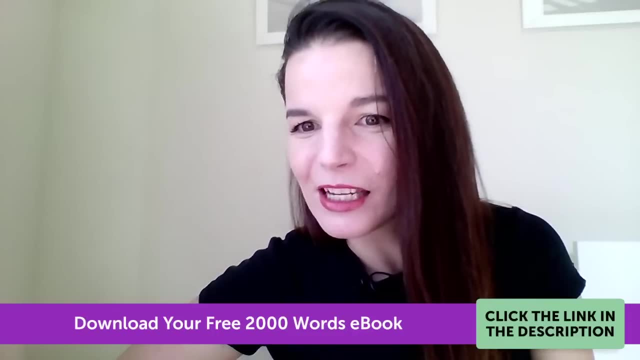 Hello Natalie and Pablo Tamalita. I am from wonderland. Okay, Oh, I remember you. You have weird comments, Don't you? Yeah, I remember Lucas. What's up? Uh, let's see Moji, Hey. 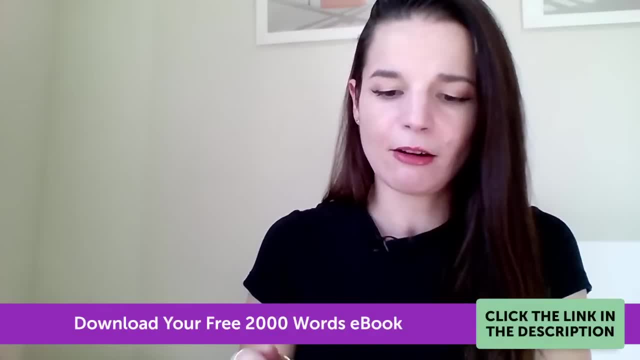 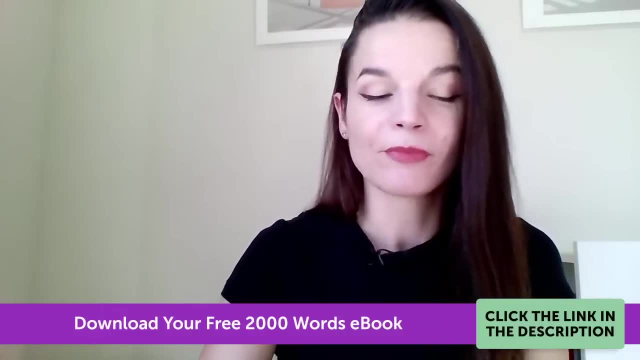 Hi everybody, Facebook, Are you here? Hey, Facebook already. Facebook, Yeah, Good Okay. Israel, Hi Jesu, What's up? Rosa Juan? Hey, Good Okay, Everybody is here. I'm going to. 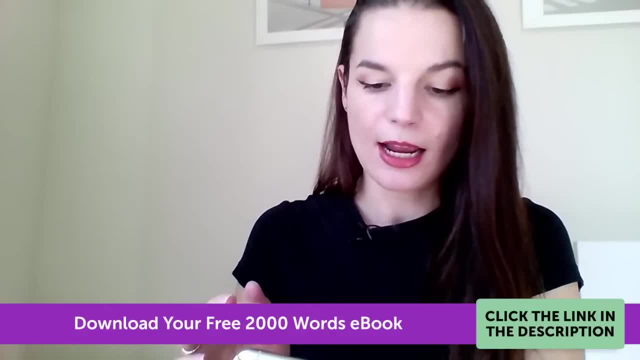 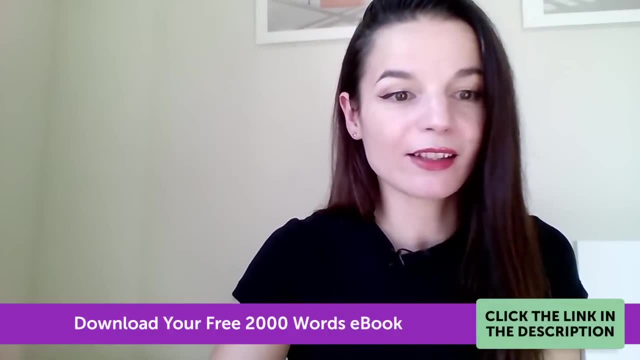 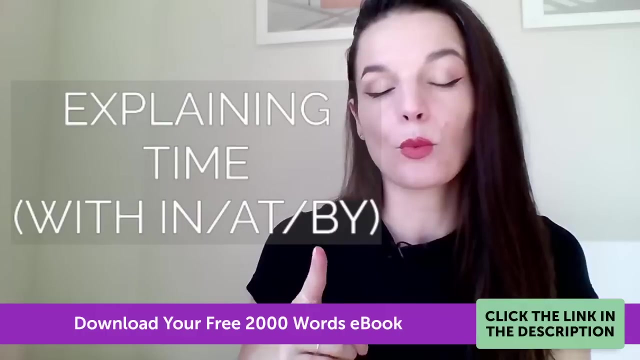 like the video now and share it. Okay, Awesome. So let's begin. As I said, today's video, today's live lesson, is about explaining time, So we are going to focus today on these three prepositions, these three tiny, tiny words that are very, very important. Okay, So they? 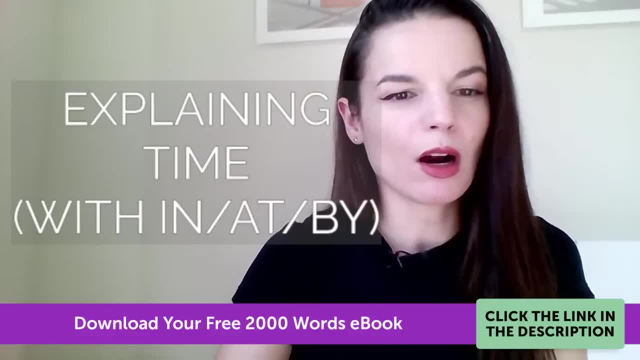 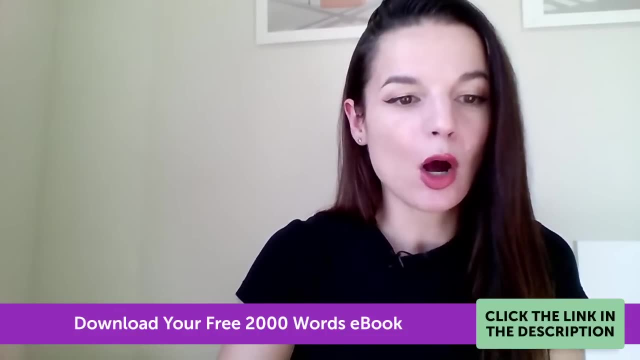 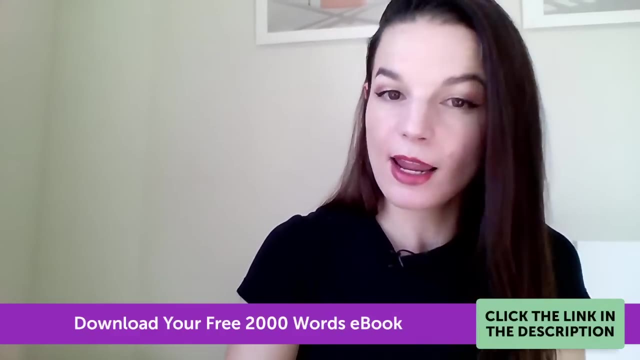 can change the meaning of a sentence. Uh, and people go: are they really? is it really that important? Yeah, they are, So let's practice them. Okay. So let's begin with the first part. for today, The first preposition we're going to look at is the preposition in time. 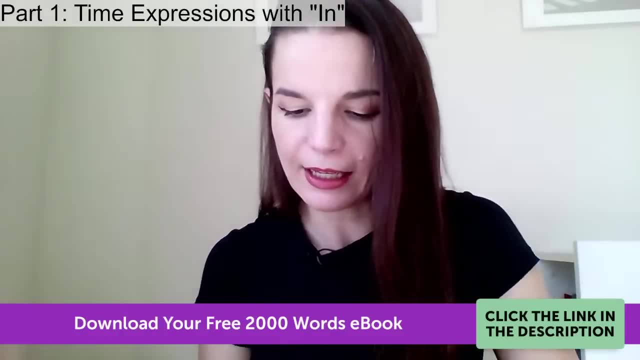 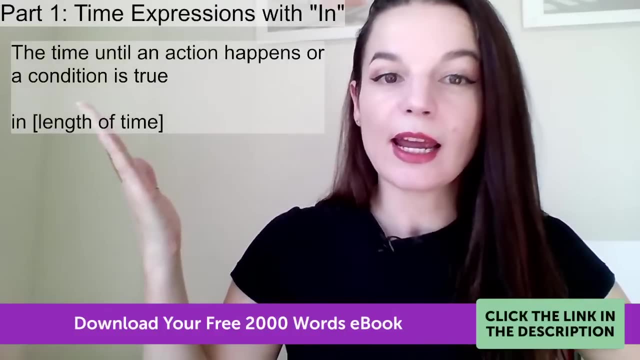 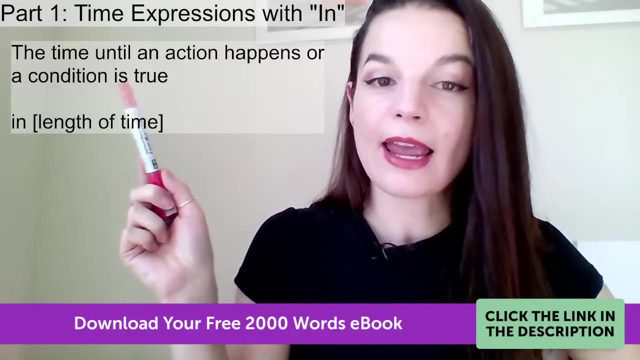 expressions with in. Okay, Let's get into it So. So when do we use in? when we are talking about time? So we use in to express the time until an action happens or a condition is true. Okay, You might think: like, what does that mean? I'll 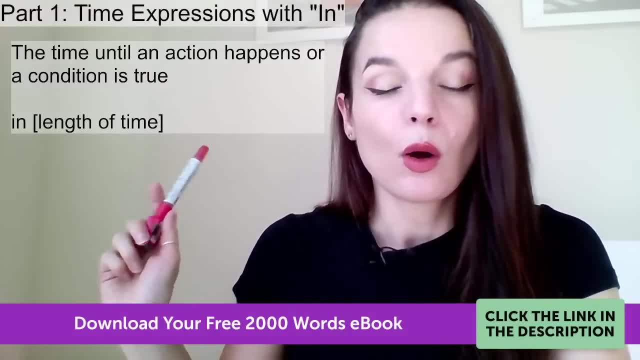 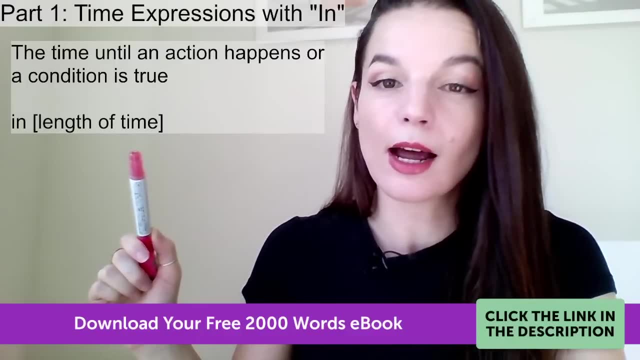 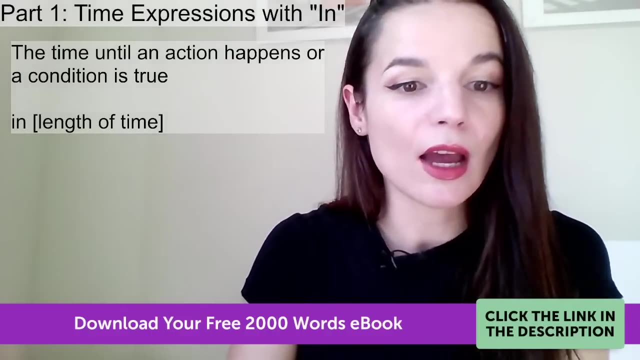 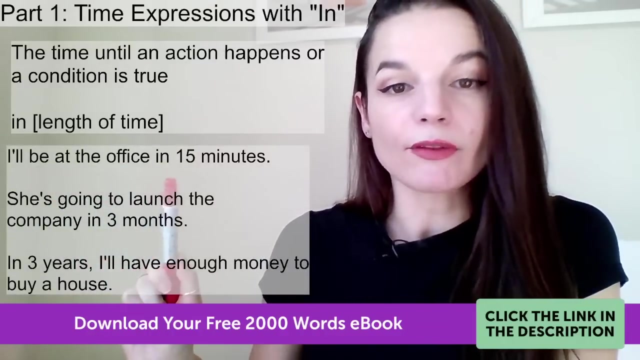 show you some examples in just a moment. Okay, So when we use the preposition in, we use in plus a length of time. This is important. Okay, Length of time goes here. So let's look at some example sentences and then we'll break down what's happening. Okay, So, first one: I'll be at the office. 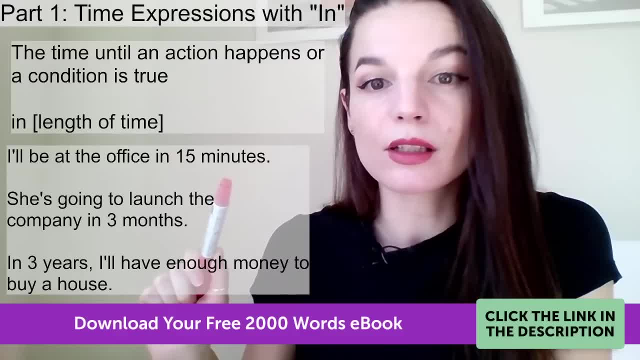 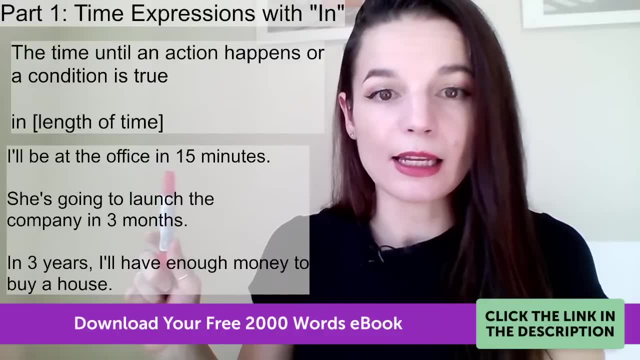 in 15 minutes. I'll be at the office in 15 minutes, Okay, So what is happening here? Here we have this in first of all, our uh in a preposition, and then we have 15 minutes. 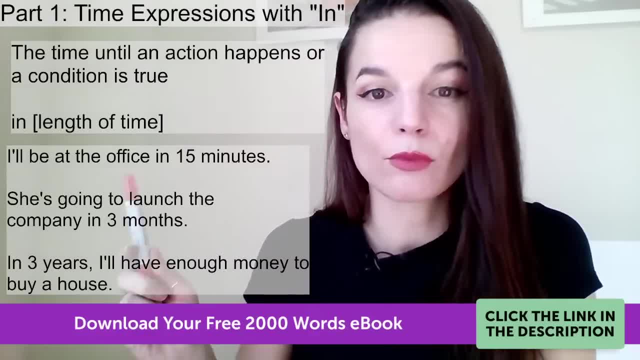 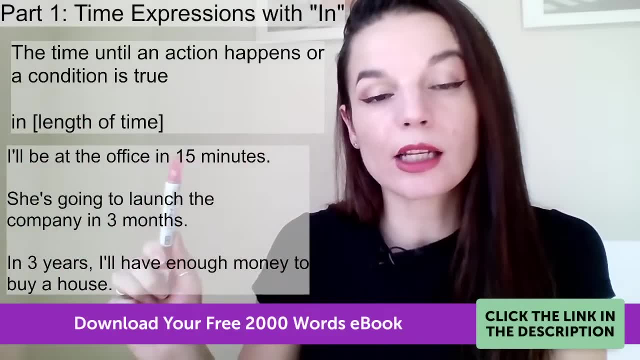 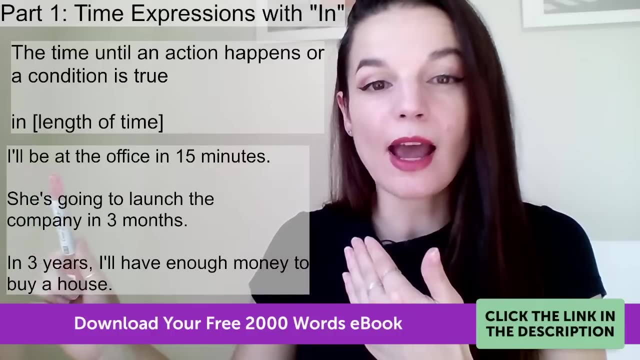 So this is a length of time, right. This is how long the time period is right. And then here is the action or condition: I will be. so this is the reduced form of I. uh, I will right, I will be at. 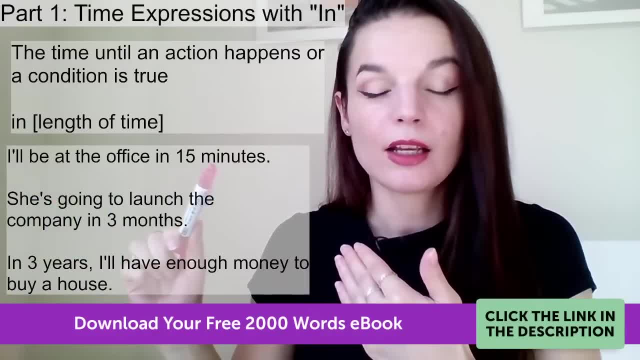 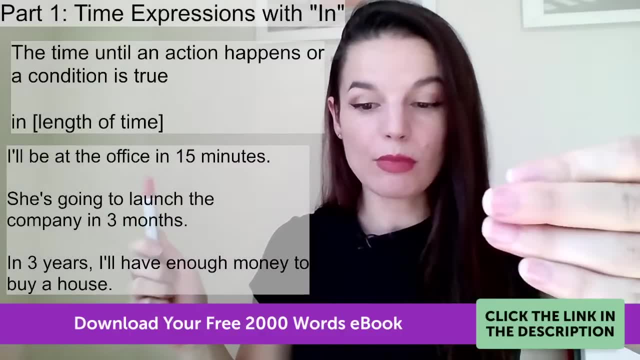 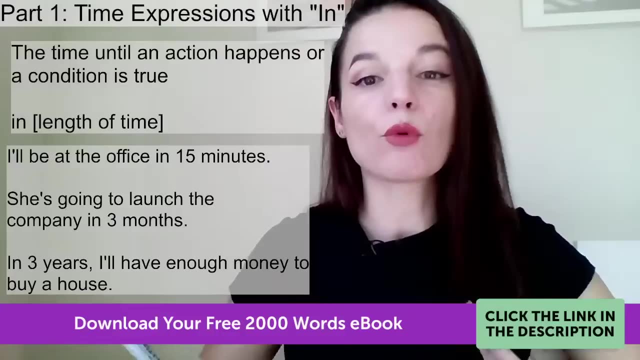 the office in 15 minutes, right? So if now it's 1230 and I say this, that means at 1245, I will be at the office, So in 15 minutes. so at the end of that 15 minutes I will be at the office, Okay, So this: 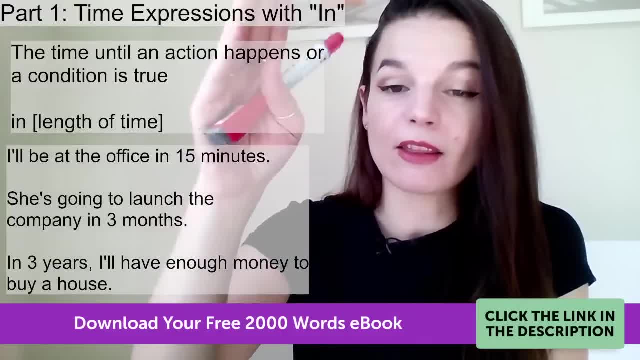 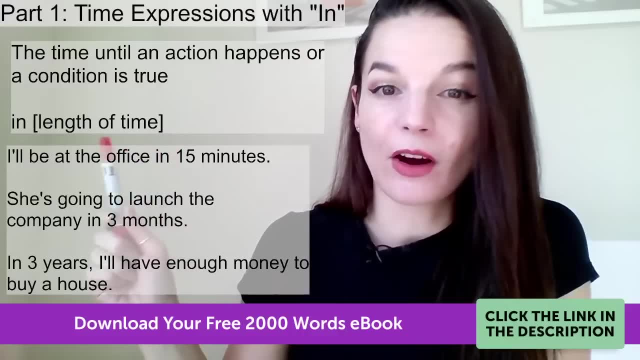 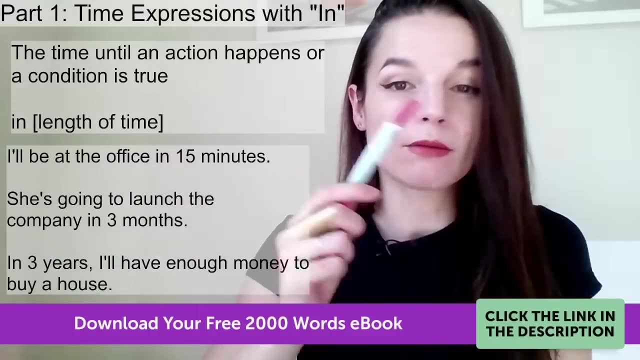 expresses when that thing or the time, the future time, the action is going to happen. Yeah, After a length of time. Okay, This is very important to a length of time. We cannot say I'll be at the office in three o'clock. Nope, Can't do that. That's stay for part two. Okay, So we cannot use. 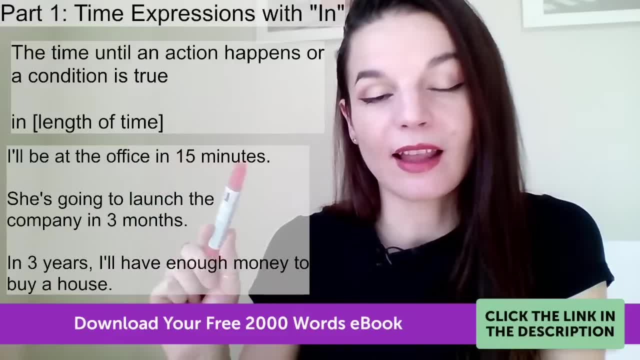 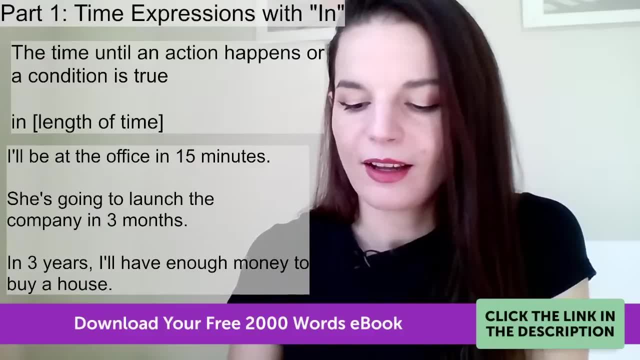 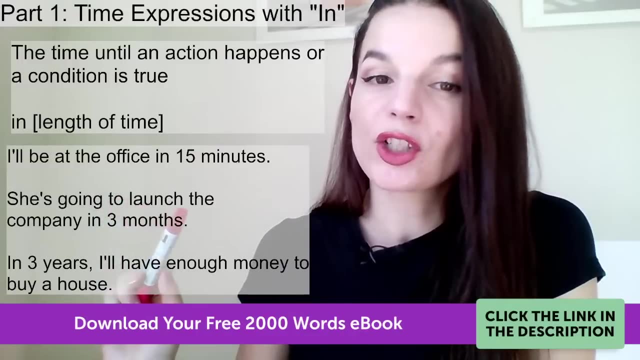 a different um preposition here with this length of time And we cannot say a time point here. Okay, So you can send your examples and I will try to check them live. Okay, For now let's continue. Second example sentence: She's going to launch the company in three months. She's going to launch the. 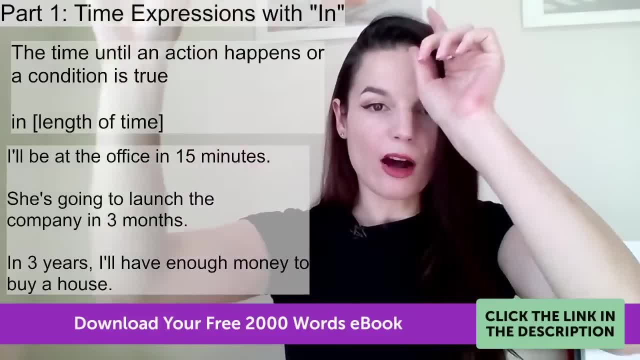 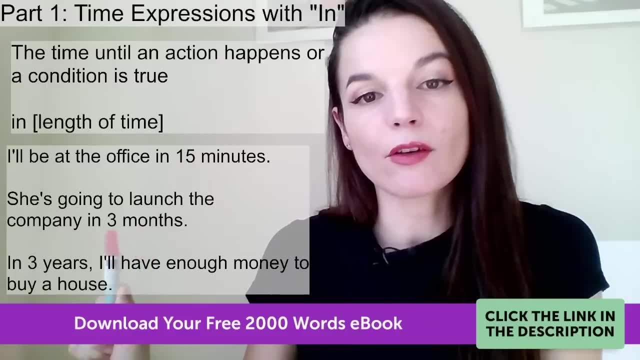 company in three months. Okay, So launch means like start kickoff, right? Okay, So she's going to launch the company in. So here's my preposition in, and here I have three months. three months, Here's my length of time. 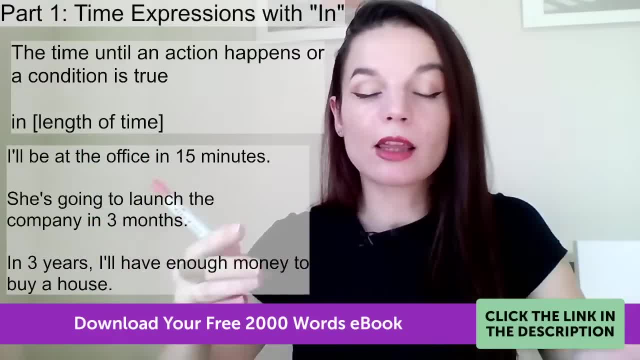 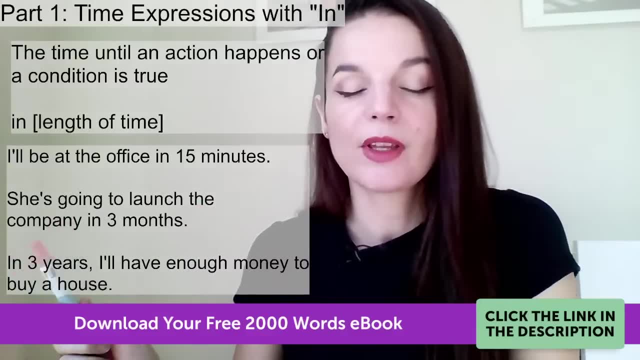 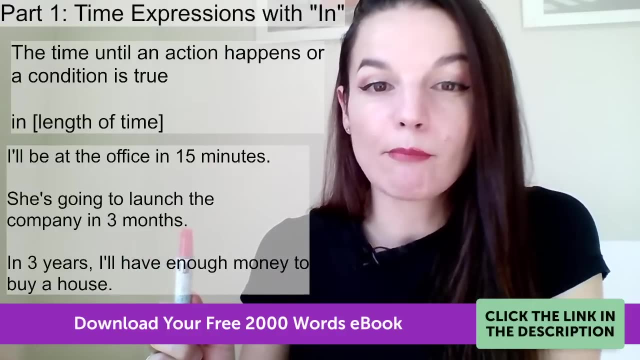 Yeah. So this months shows me the period until this happens going to launch the company. So future tense sentence: Yeah, Okay, So again, we have to use this time, uh, this length of time- Important point: I noticed many learners forget this. S at the end: three months. 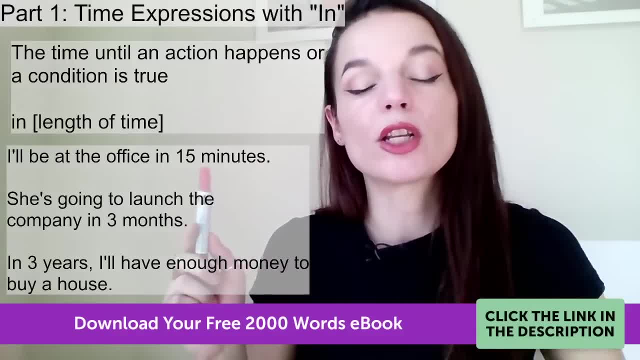 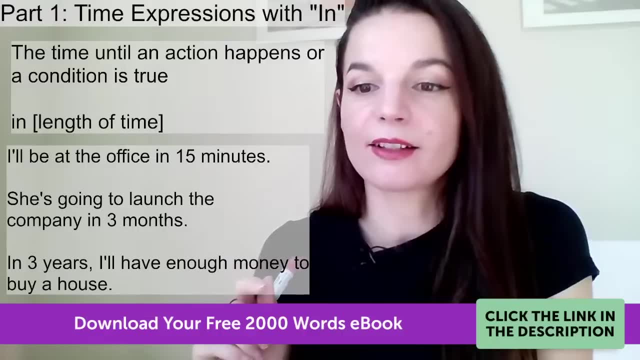 Or 15 minutes, Make sure it's a plural. When you have a countable noun like minute or month, make sure you have that S at the end. Okay, All right, Let's go to the last example, And then I: 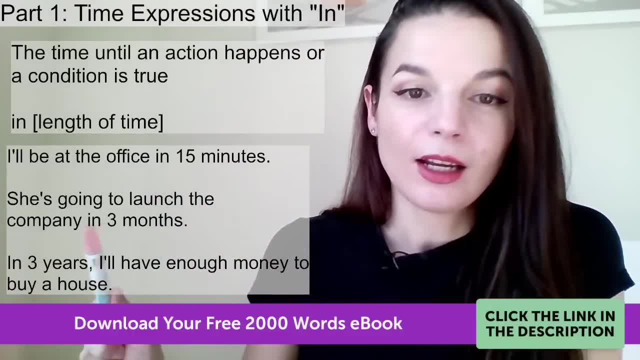 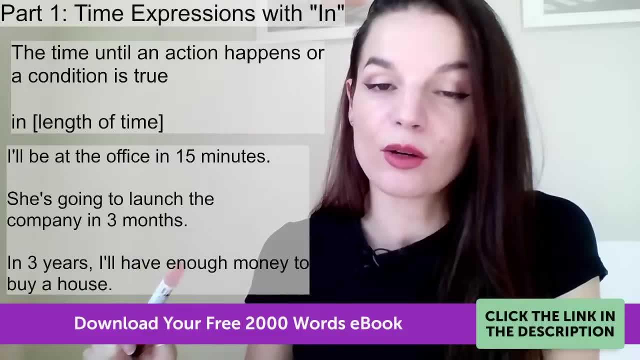 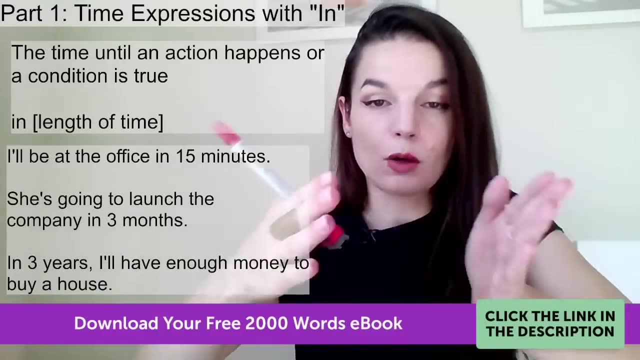 will come to the chat for your examples. So here I have it at the beginning: Yeah, In three years I'll have enough money to buy a house. in three years I'll have enough money to buy a house. So here in three years, So in this length of time. so after three years, right, I will have enough. 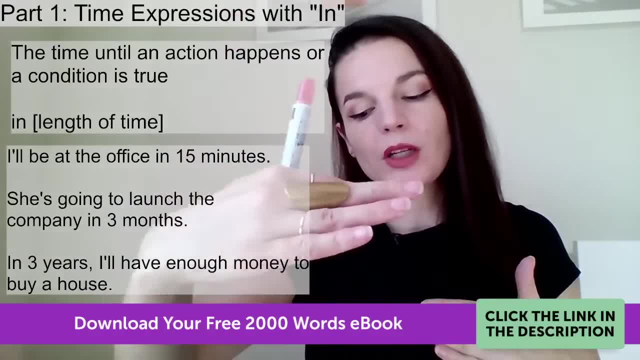 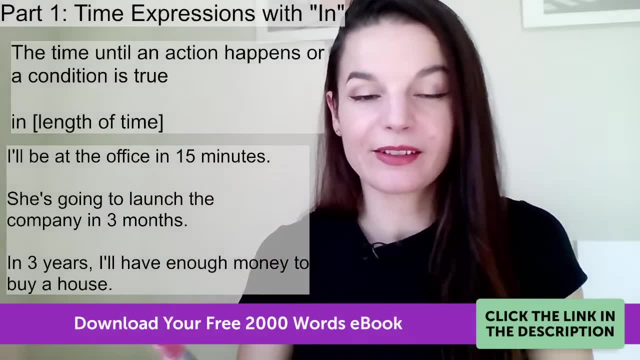 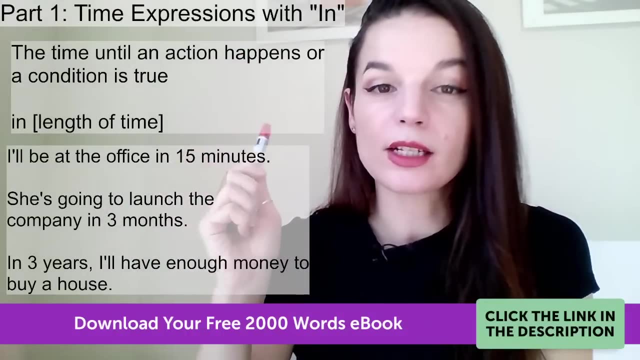 money. So in the future, in three years, three years from now, my condition will be enough money right To buy a house. Okay, So we use in to talk about this time until that thing happens or until the condition is true. Okay, 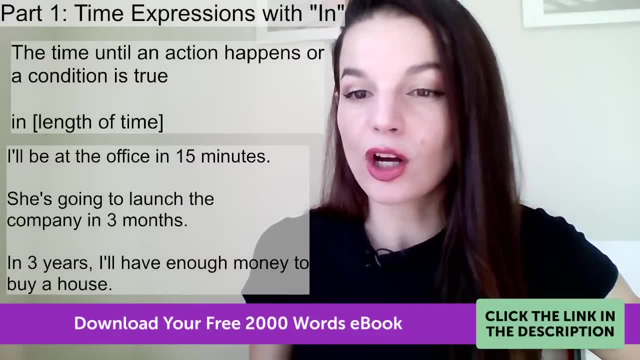 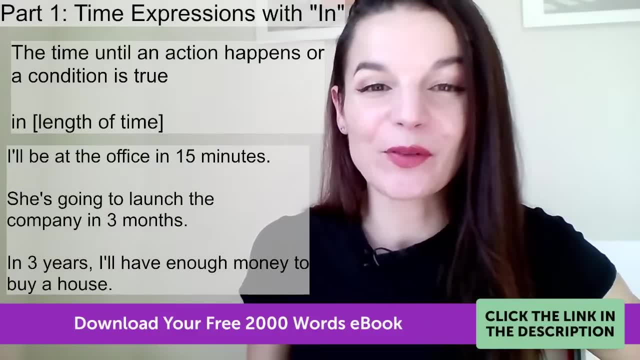 All right, I'm going to come and check your example sentences now. Gospel said I'm going to school in the morning. Great, Yeah, Okay, Oh yeah, I didn't talk about this today, but in the morning, in the afternoon and in the evening we also use that to talk about it, Okay, 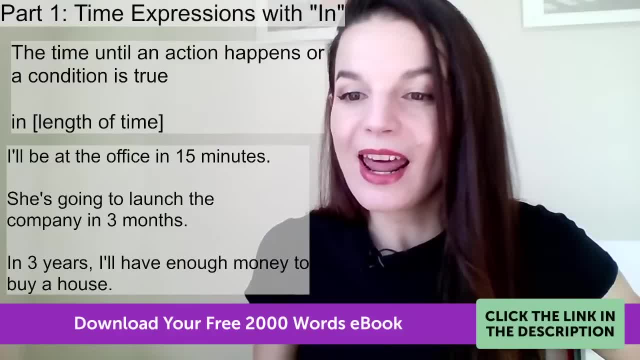 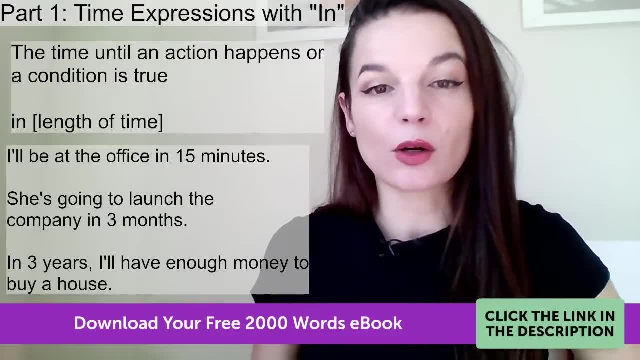 Gustavo, one of our members, hey says I'll get a pizza in 30 minutes- Great, Nice, Okay. Patrick wrote: I'm going to have lunch in 15 minutes- Nice, Perfect, So in 15 minutes. 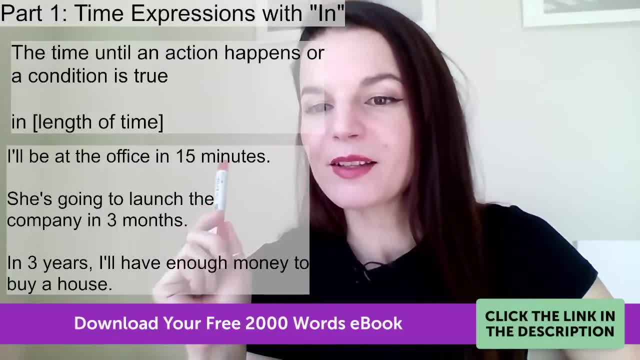 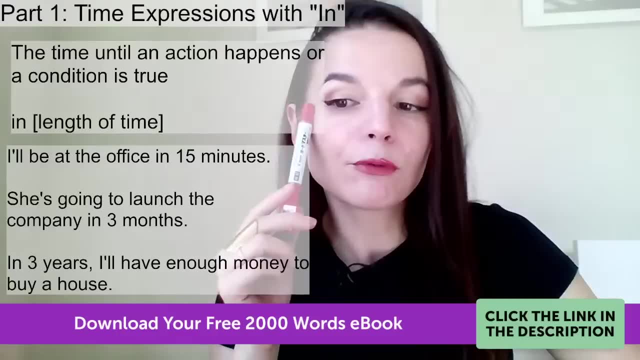 Great Great Marlene wrote: I'm arriving in 30 minutes- Perfect, Nice job. Marlene Obeid wrote: I work in Walmart. Oh, past tense maybe, or I'm not sure, I have worked in Walmart. 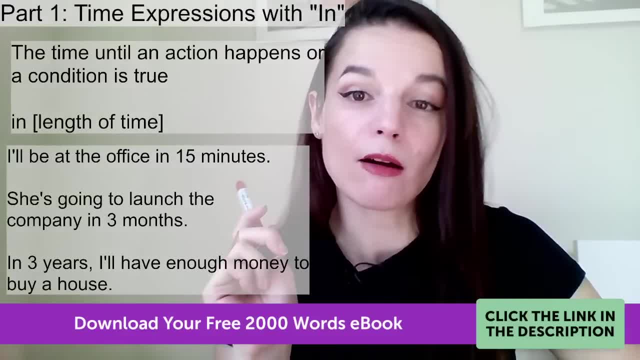 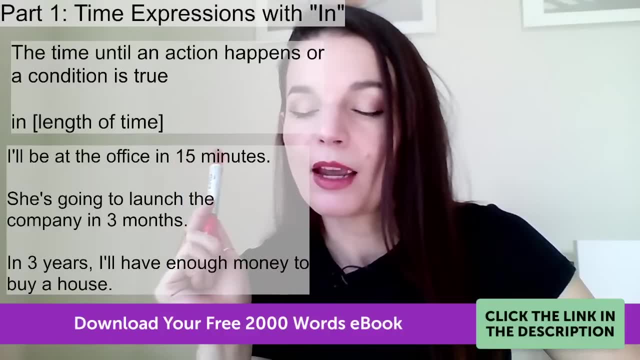 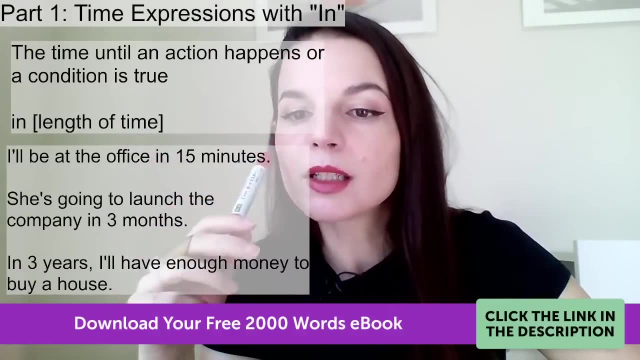 for three months, or I worked in Walmart. Do you work at Walmart now? I have worked, Yeah. If you do not, no longer. I worked at Walmart for three months, Okay, You use the location in? I work in? Yeah, Okay, Others. I'm looking for examples. 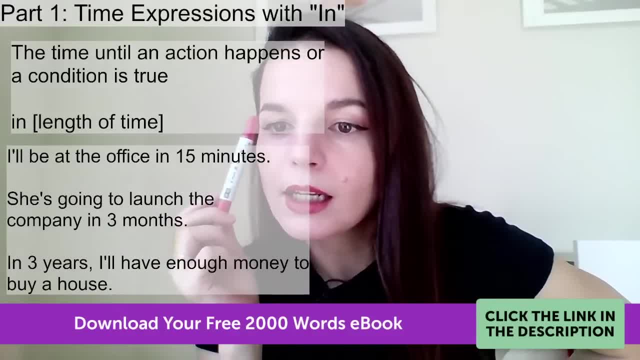 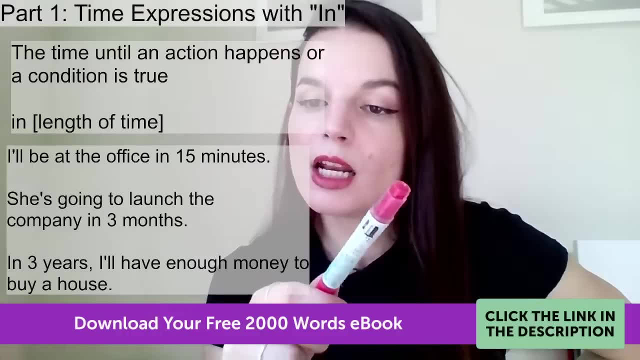 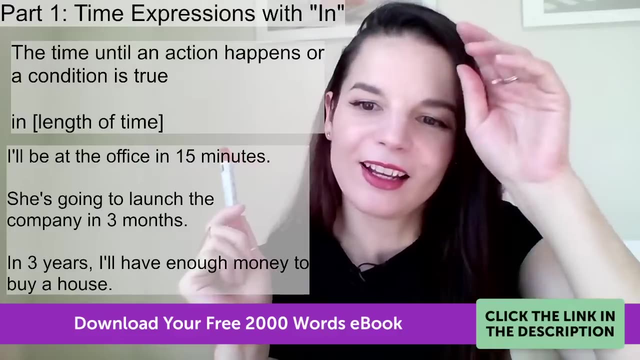 And let's see. Well, hello to everyone saying hello. The Black Eagle wrote they'll play the final soccer match in one month, Nice, Okay. Michaela Velasco wrote I'm going to sleep in 30 minutes. Okay, David wrote I will go to bed, Was it? I will? Just I'll? Yeah, I'll go to bed. 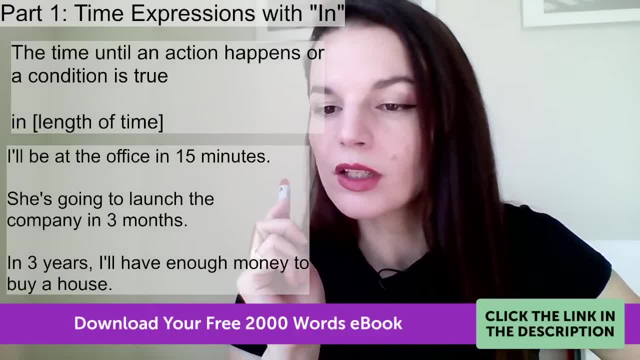 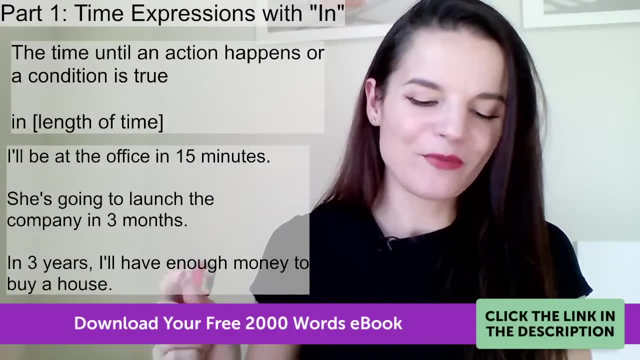 in 10 minutes, Okay, And Ninad wrote: I'll be at the office in 30 minutes. Good Facebook, what you got? Facebook, Hello everyone. Examples: There's one, Rosa, I'll be right back in two. 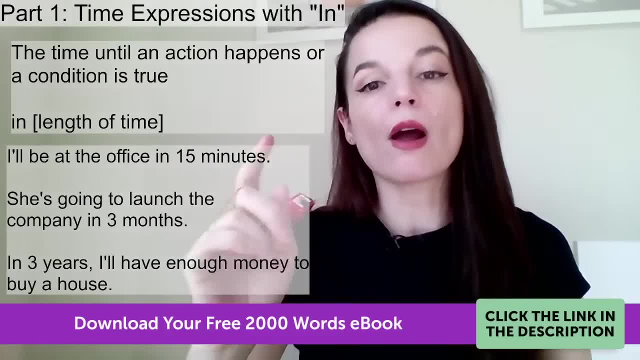 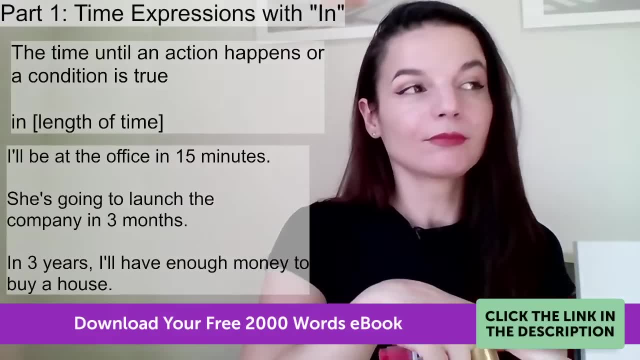 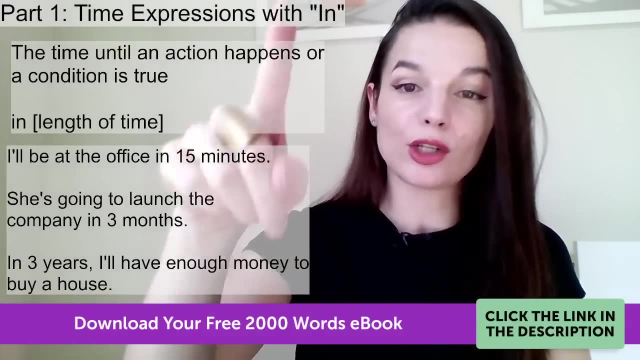 hours. You don't need to put right back in two hours. Also, right back sounds like very quick. Two hours is not right back Generally. I'll be right back, Leave, finish, finish. the sentence there Means I'm coming back in a few minutes. Yeah, So I'll be back in two hours. Sounds better. 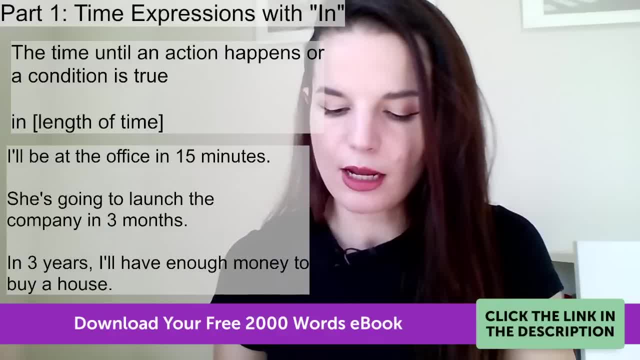 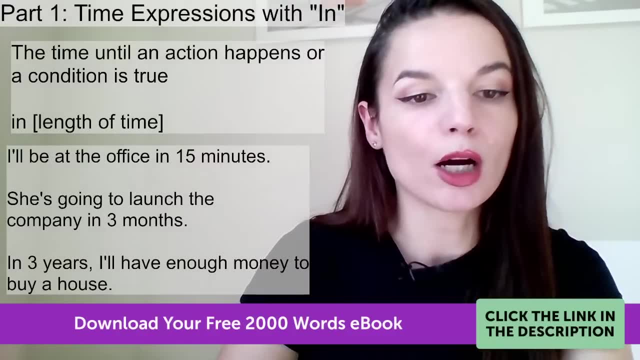 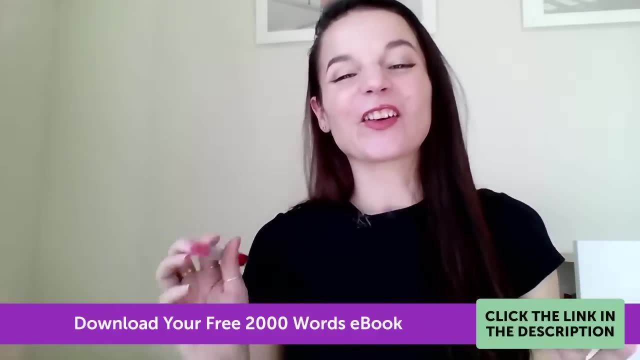 there, Juan, I will be at the university in 30 minutes. Nice ones. Okay, Sounds good In. sounds good to me. Let's take a break And then let's go into part two. We're going to change the preposition- How exciting. So, if you missed it, really really quickly. 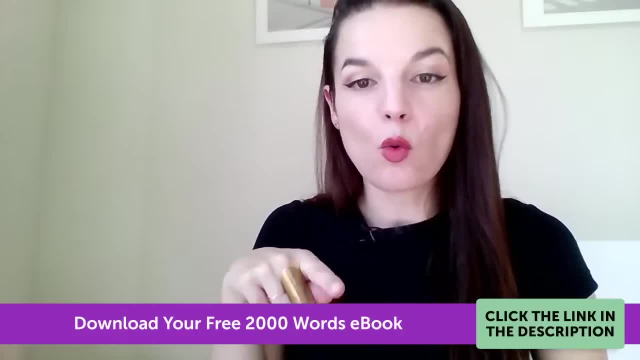 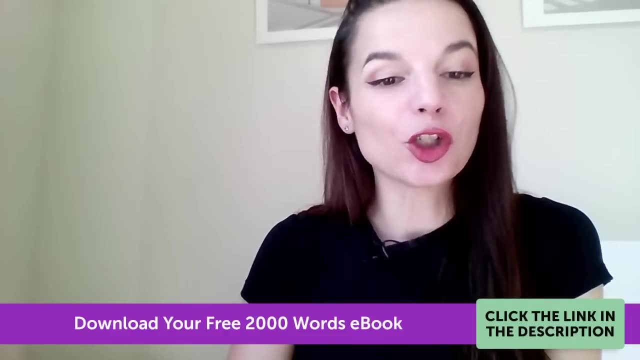 our team has created recently a 2000 word ebook that is free. So I talked about this earlier, But if you want to get this 2000 word ebook- these are the 2000 most commonly used words in English- you can do it in two minutes. So if you want to get this 2000 word ebook, you can do it in two. 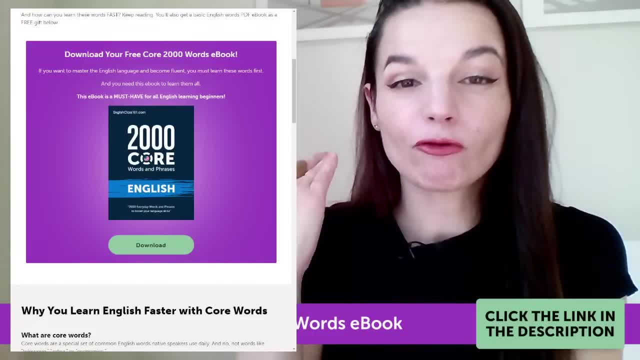 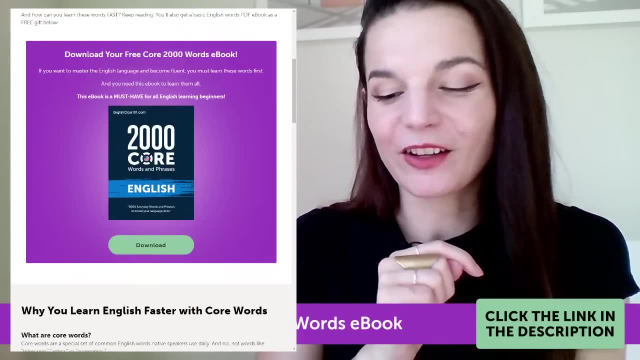 minutes. So if you want to get this 2000 word ebook, you can download this from englishclass101.com for free. You need your name and an email address. only You can find this from the link below the video if you're watching this on YouTube, or above the video if you're watching on Facebook. So this 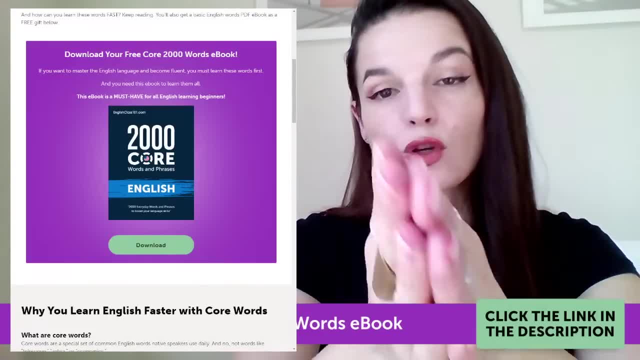 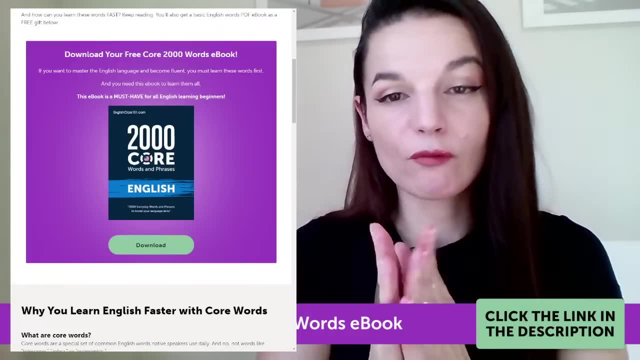 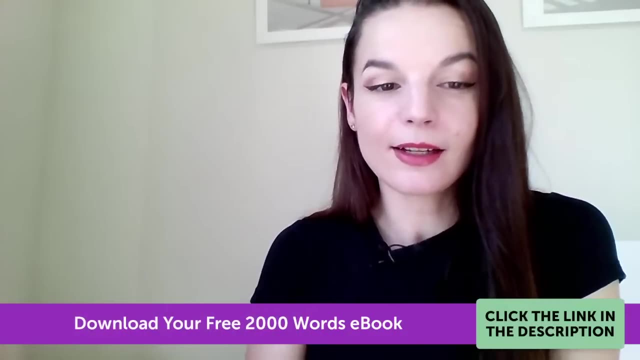 ebook gives you the most common words so you can study vocabulary efficiently. right? You study the words that are the most important words first, So check this out. I hope it helps you with your vocabulary study. Okay, All right, Let's continue to part two: New preposition. If you have not, 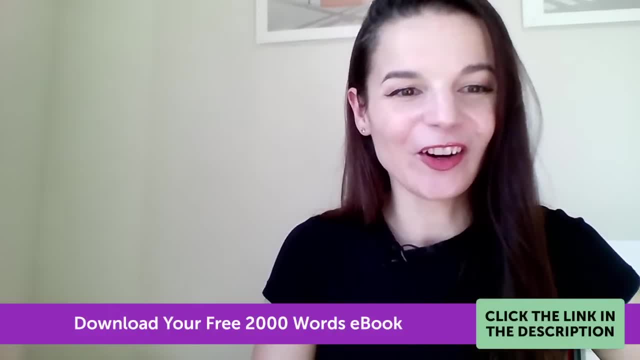 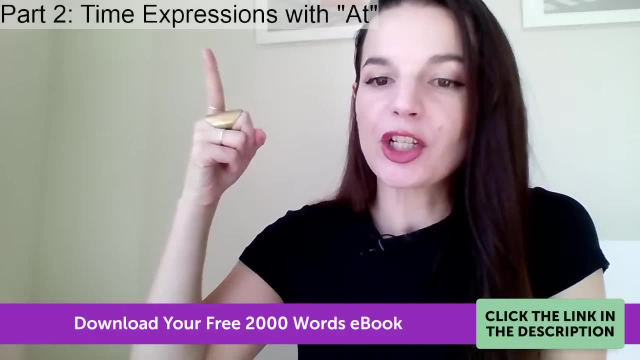 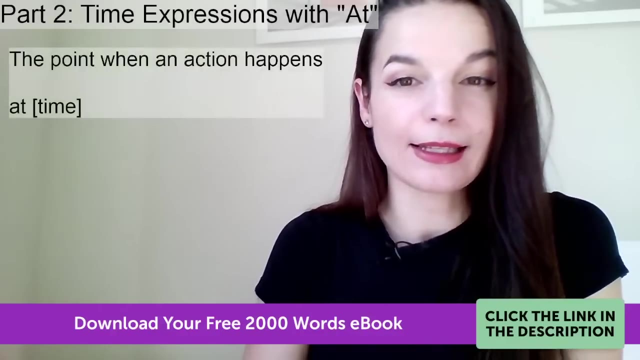 please make sure to like and share the video because it helps other people to find the lesson. Yeah, Okay, Let's continue to part two Time expressions with at Okay, At is our second preposition for the day. When do we use this guy? We use at to express the point? 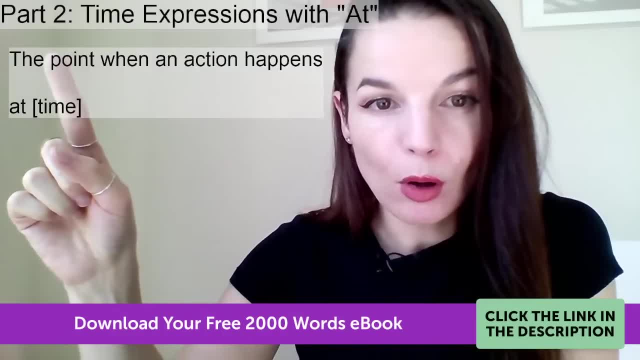 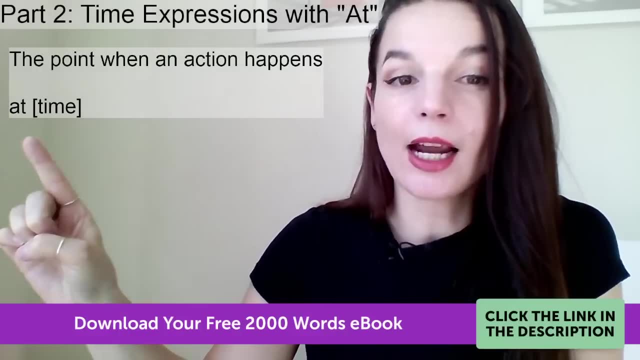 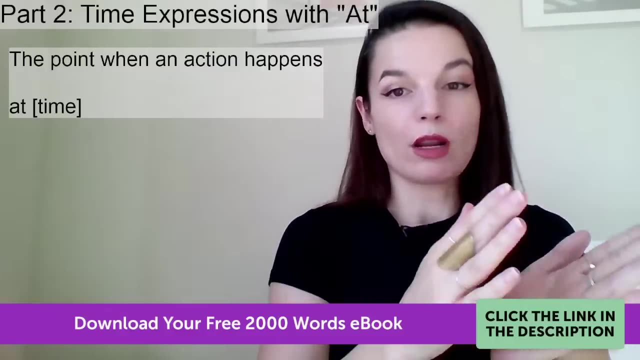 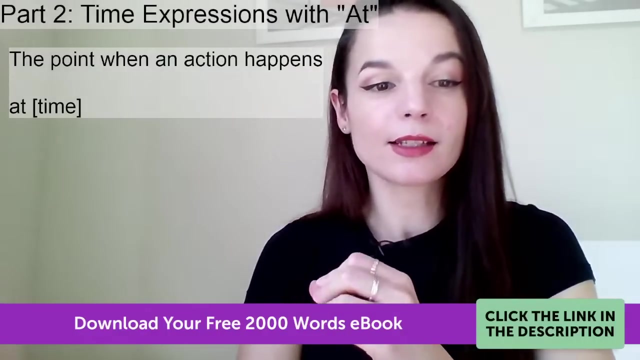 when an action happens, So point the point. So when we use the preposition at, we use it before the time. So we do not use it before a length of time Like within, we said, 15 minutes or three months, right With at. we use 2 pm, 3.30, whatever right We use at plus the time We use. 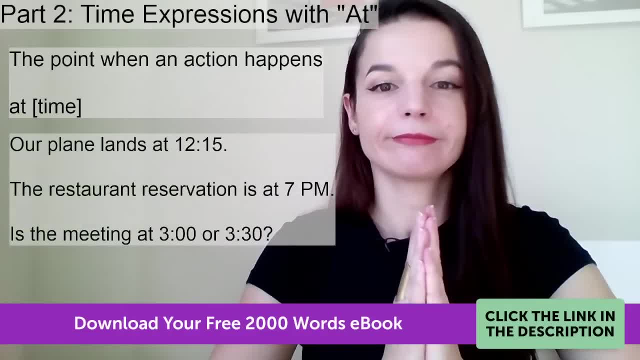 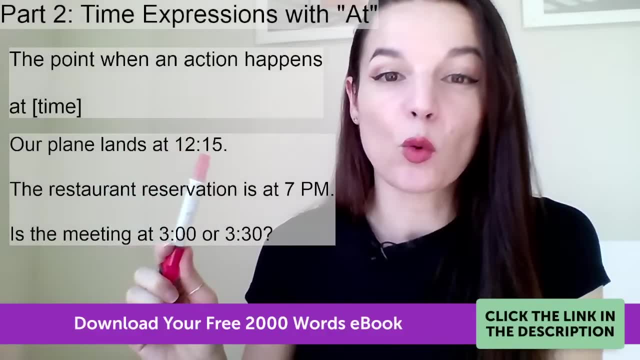 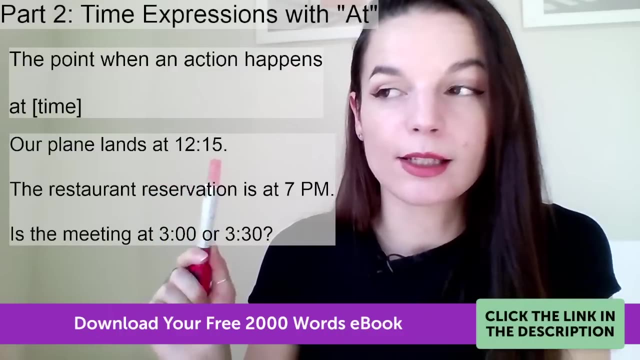 this a lot to talk about our schedule. So Let's look at some examples. Our plane lands at 12.15.. Our plane lands at 12.15.. So here we have, at plus our time, 12.15,. right, We could say a quarter past 12 as well, if we want to. So also. 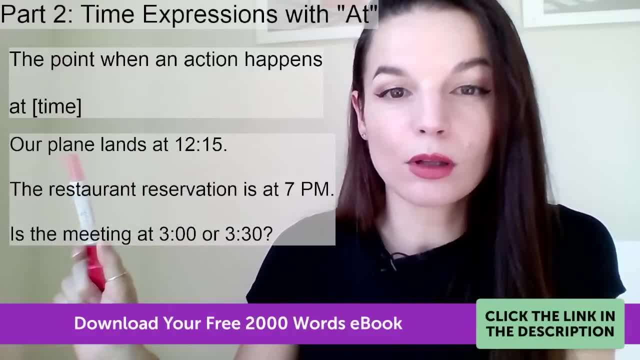 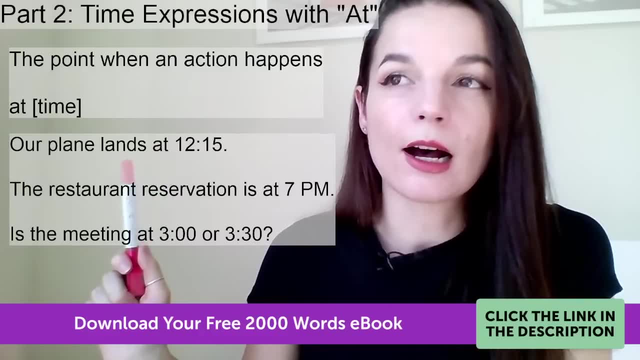 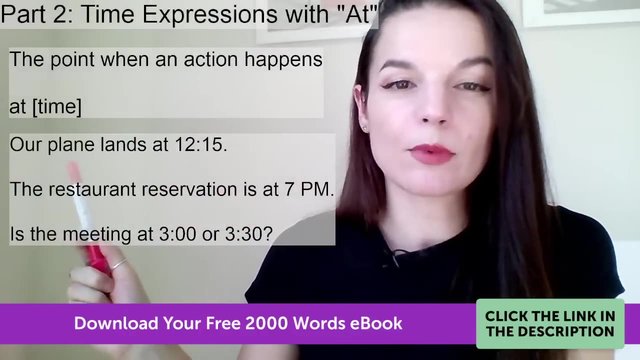 note: our plane lands. So here is a simple. this is a present tense sentence, right? Our plane lands. So a quick reminder: we use present tense to talk about schedules- bus schedules, train schedules, plane schedules- right? So sometimes I 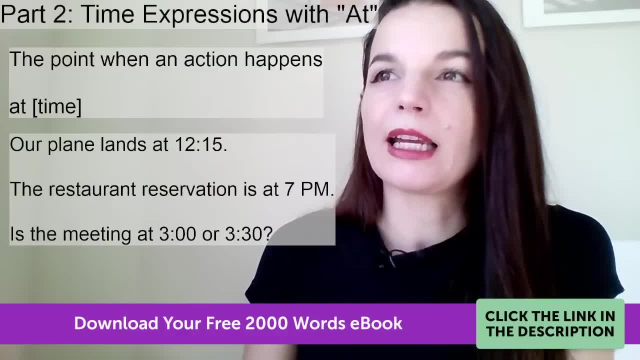 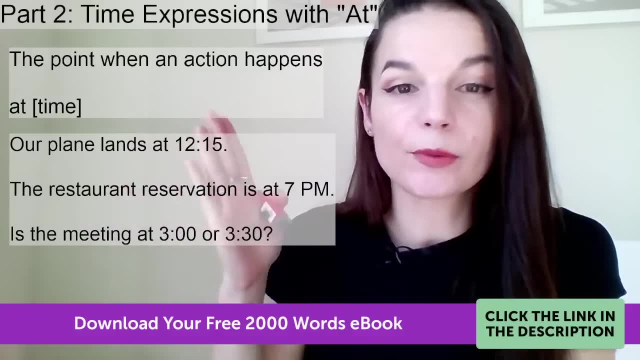 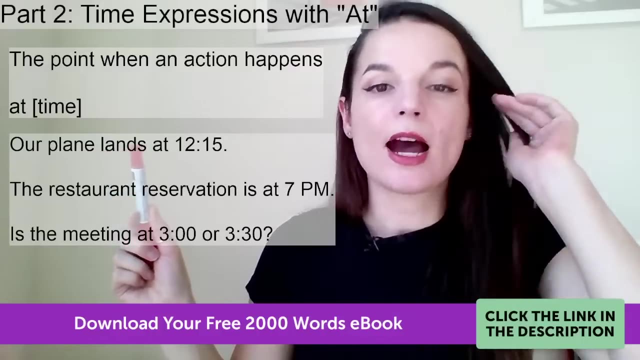 see learners write something like our plane is landing. I suppose that's okay in this case, but we use this to talk present tense to talk about schedules a lot, So you will often see present tense used to talk about these kinds of things. okay, Our plane lands at 12.15,. okay, Let's. 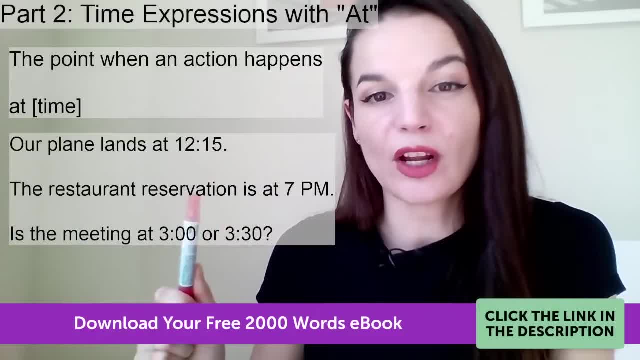 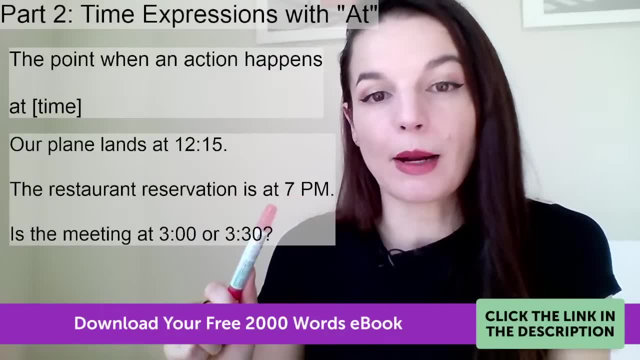 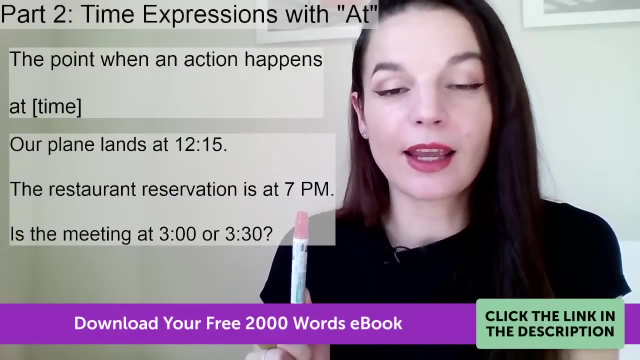 continue to the second example. The hotel reservation is at 7 pm, The restaurant reservation is at 7 pm. So here's my at At plus my time, 7 pm, 7 at night. So again, this expresses the point when an action happens or when something is. 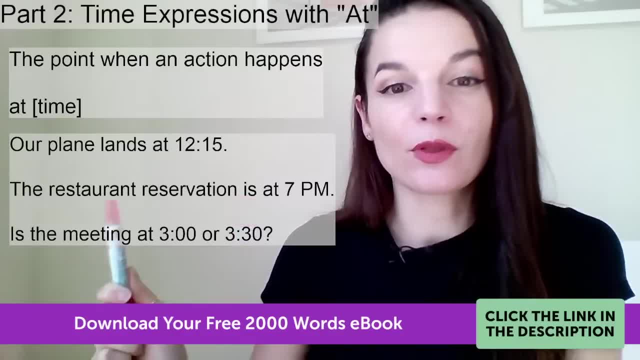 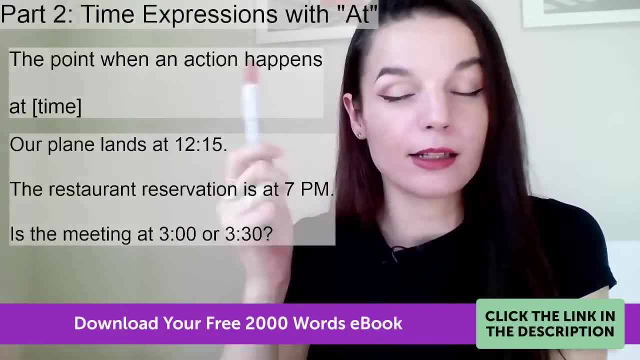 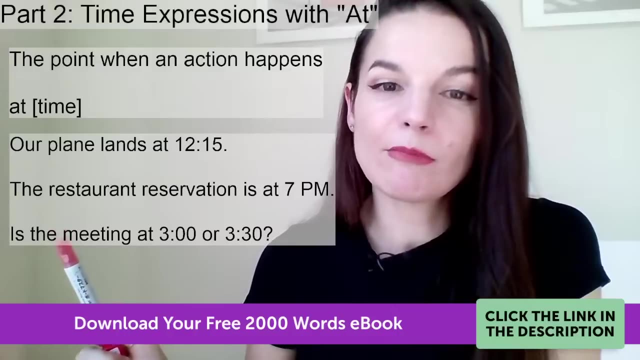 true, The restaurant reservation right. So this is the scheduled item. The activity we have at 7 pm in, not on, I don't know, at 7 pm, okay, And finally, is the meeting at 3 or 3.30?? 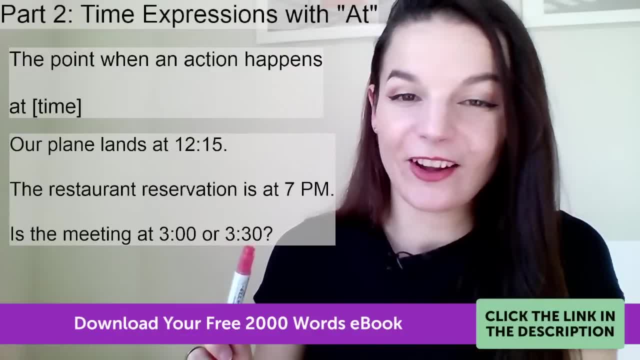 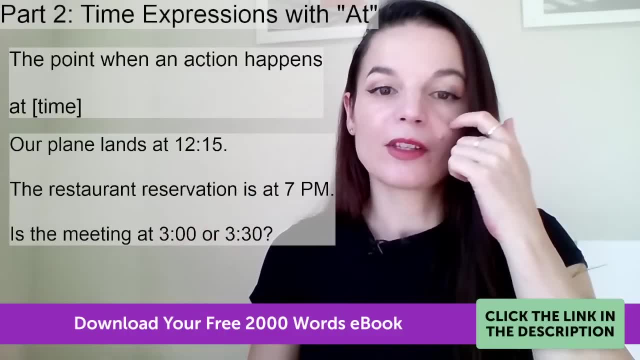 Is the meeting at 3 or 3.30?? You could use at again here if you want to, but we know that it's a time We can use this at for this and for this. It's easy to see, So you could say: is the meeting? 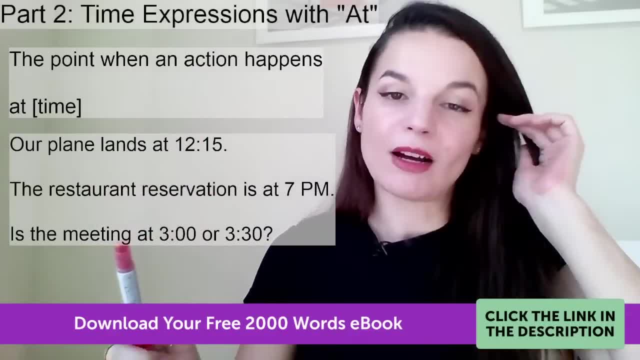 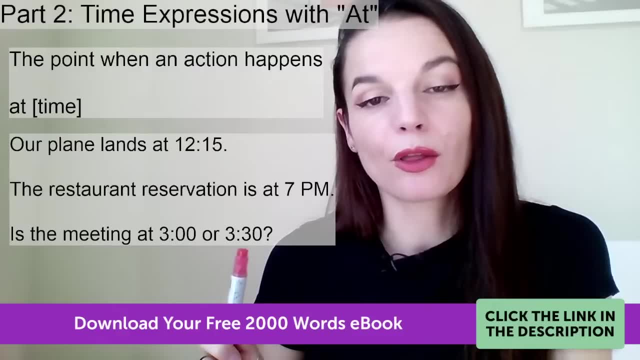 at 3 or at 3.30? That's okay too, But for efficiency we can use it just once, okay. So again, we have this before the time, 3 or 3.30, okay. So the key here is with at. we use it with. 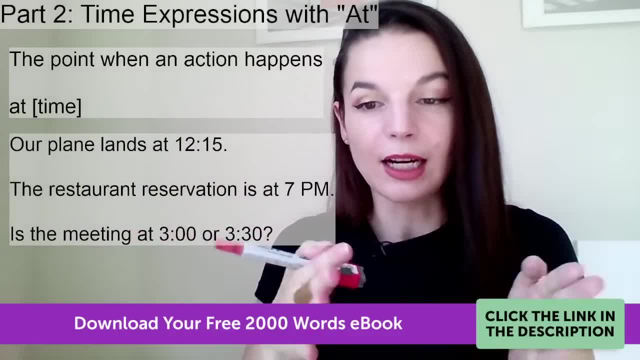 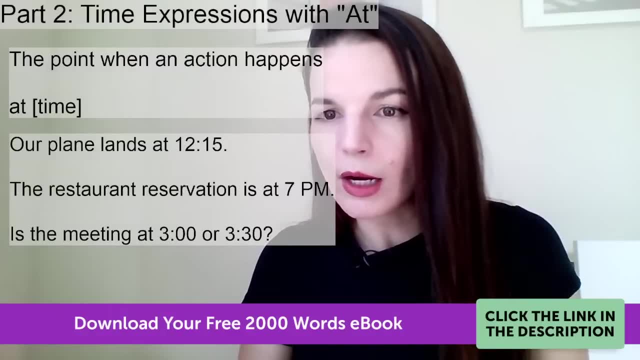 a time In. we use with a length of time, a duration, here. okay, Let's take a look at your examples. Let's see. I'll come to YouTube first. Someone sent. why is someone sending a bunch? oh, I thought those were snails. It's an emoji, It's not. 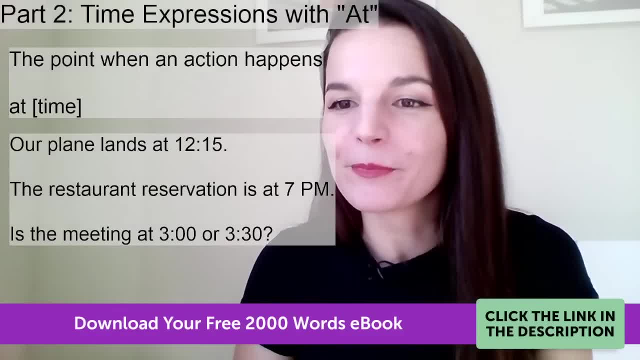 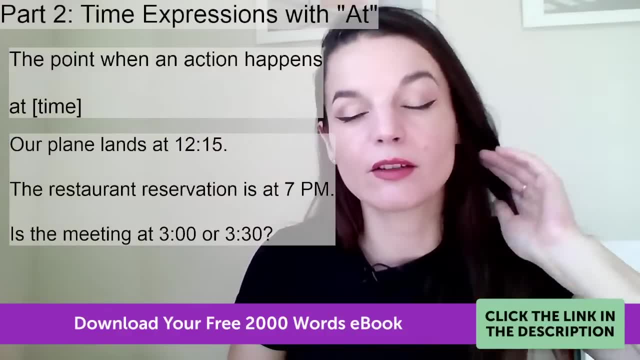 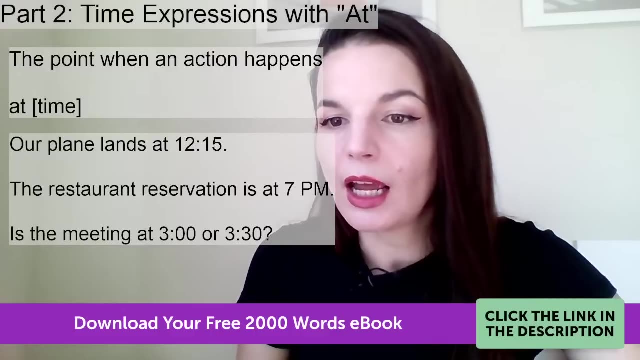 I couldn't see It's very bright here. Okay, Let's see. I'm looking for time uses of at. Some of you are sending location location uses Different from today's lesson. yeah, Michaela wrote English classes are at 8 am with Alicia. Perfect, Very nice one. Obaid wrote the soccer. 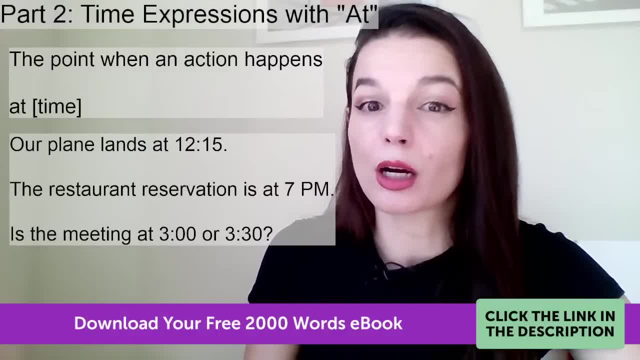 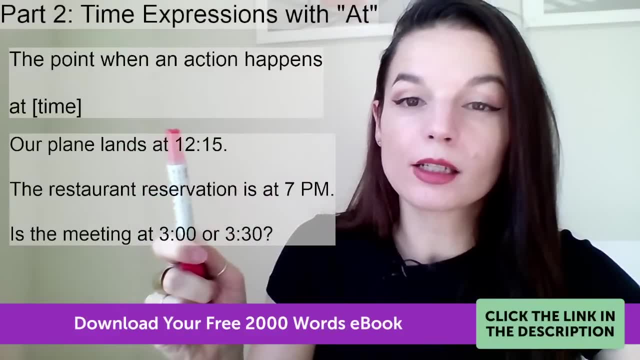 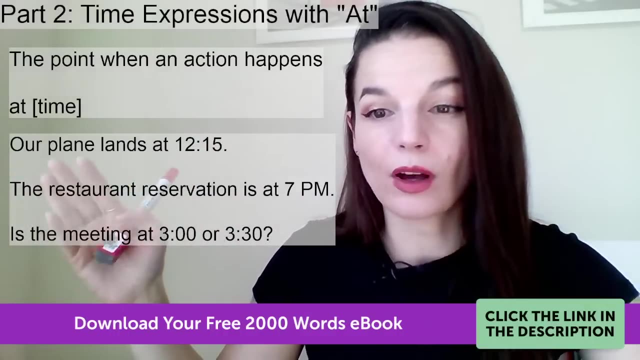 end at 7.45.. So the soccer- maybe the soccer match or the soccer practice, not sure- Ends same as lands. yeah, End in present tense is ends. It ends. Class ends, Practice ends. The match ends at 7.45.. Yeah. 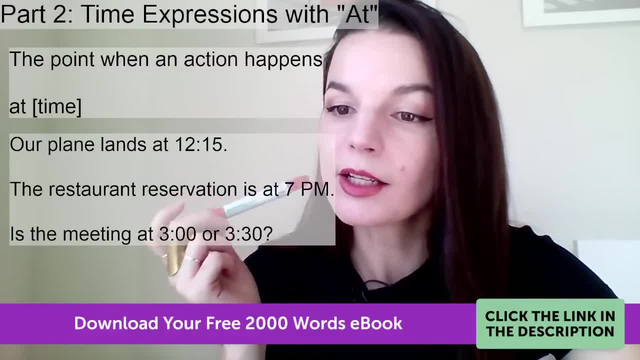 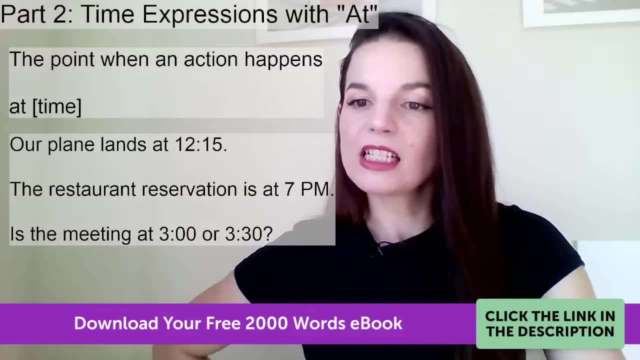 Then it's perfect. Natalie wrote we start our lunch meeting at 1 pm. Nice- Okay. Max wrote the concert will start at 16.15.. Nice- 4.15.. Okay. Ninad wrote. my friend was going to come. 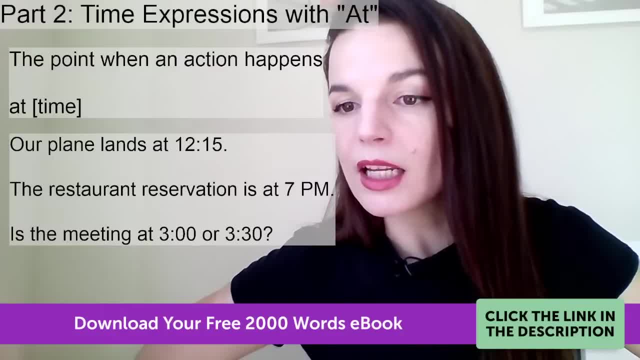 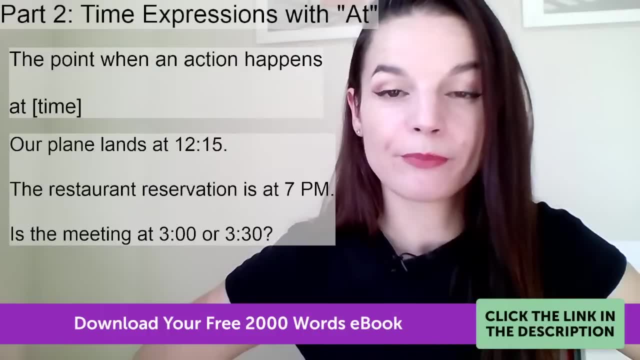 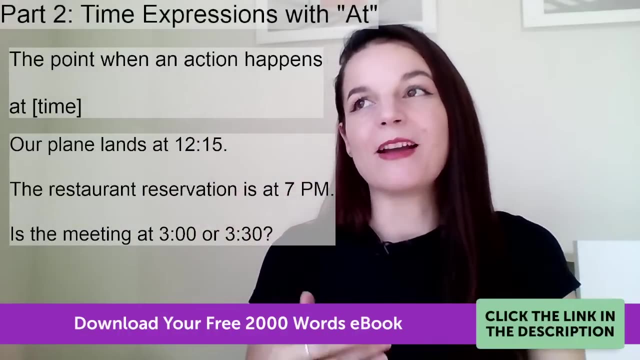 at 7 pm. Perfect Miguel wrote: I'll have an English class at 10 pm. I would say I have an English class. I have an English class at 10 pm, Like it sounds like a fact, right, Instead of I will, which we use for like decisions we make, Maybe. 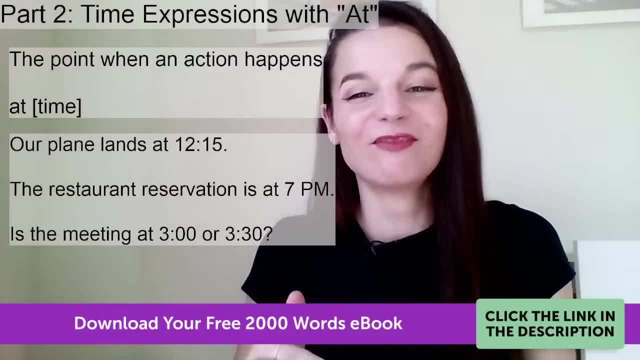 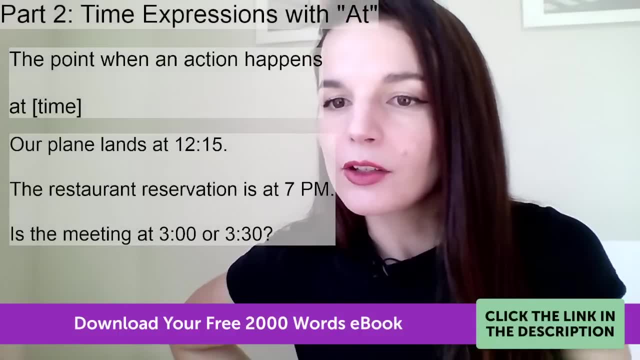 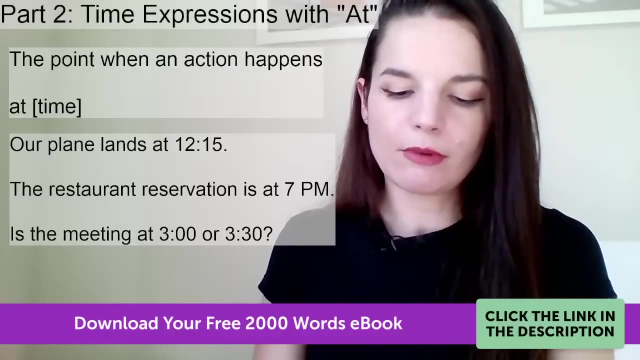 you're choosing now. I'll have an English class at 10 pm. Maybe it's like an online menu, I don't know. Usually we say I have, I have. Okay, Gustavo wrote my dentist appointment is at 4 pm. Okay, Facebook, I didn't forget about you Facebook. do you have any examples? 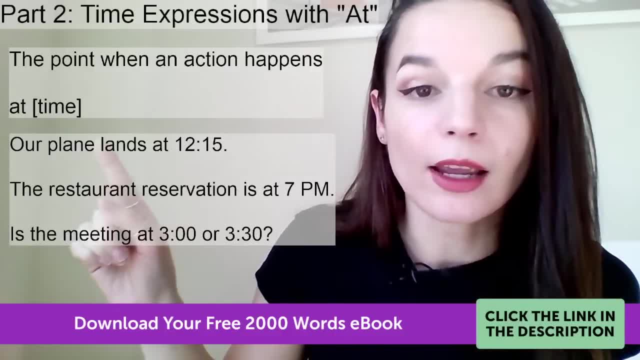 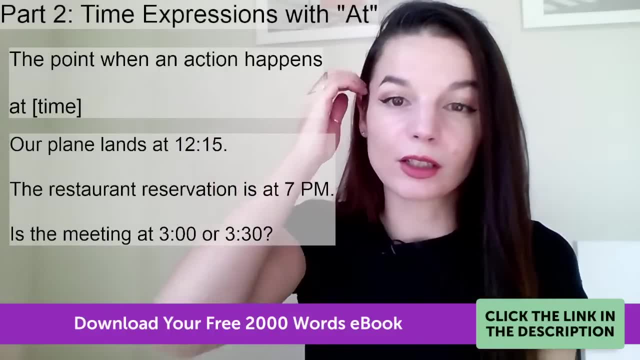 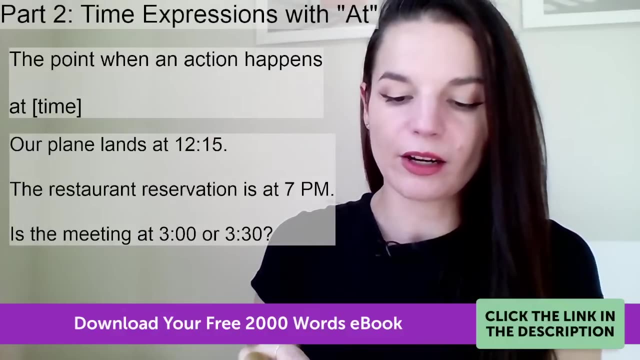 Rosa said the Kentucky Fried Chicken arrives. Okay, I've seen a few of you miss this S Yeah Present tense S Rosa, that's one for you. Someone. I mentioned it earlier, Obaid, I think it was on YouTube. Don't forget your S Yeah. Salman wrote. the game will start at 5 pm Nice. 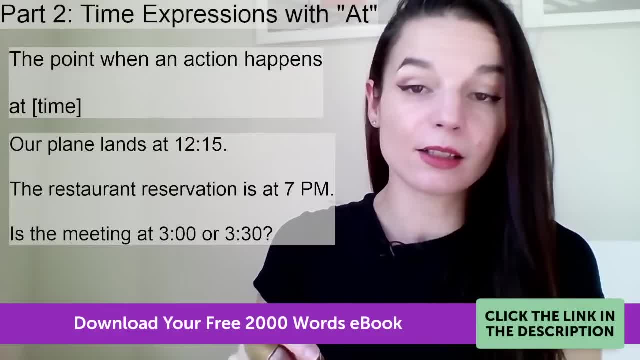 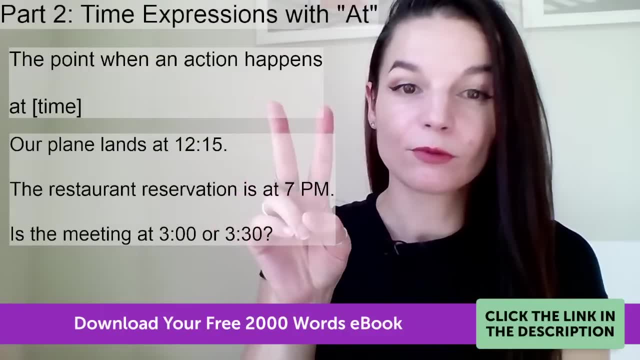 Okay, Tyson said. she said she is. she's going to meet at a place she chose, in at 5 pm. You have two prepositions. Which do you think is correct? You have in and at next to each other. there You can send. 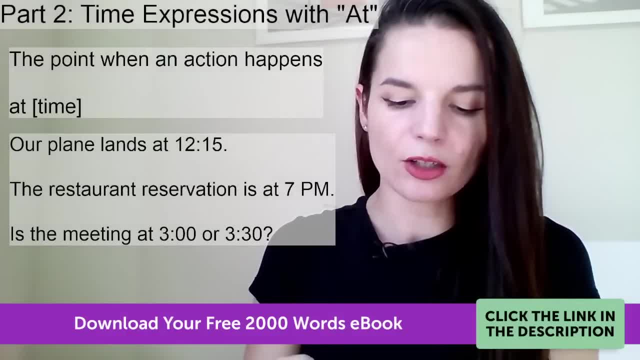 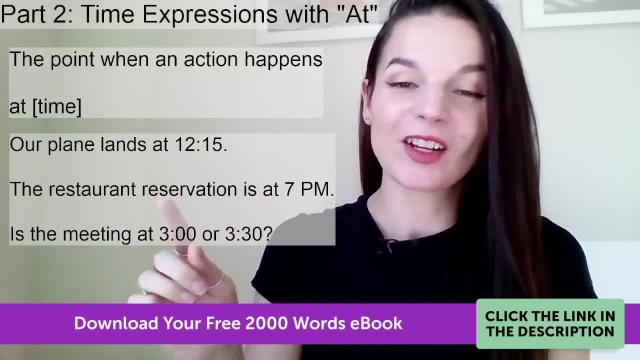 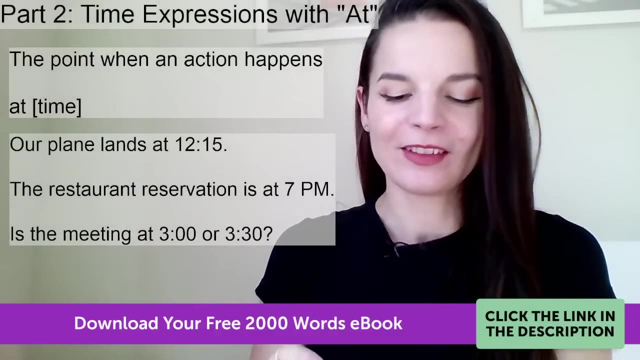 your example again: Tyson, Glenda, your English class start at 9 pm. Glenda, you have the same S problem: Starts, Your English class starts. So some of you, after this lesson, your homework is to search my present tense lessons on YouTube. Yeah, Starts, Right Starts. 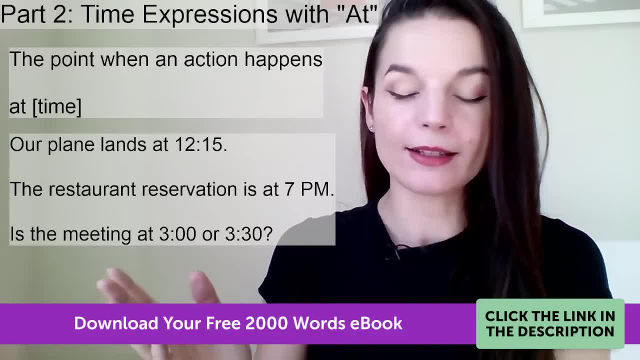 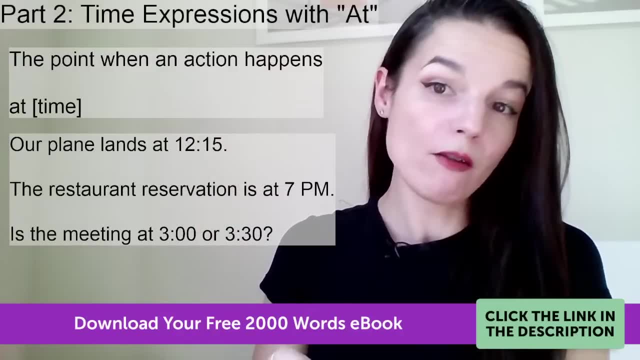 Okay, Lita, my cousin is what at 10 am My cousin, so you have no verb there. My cousin is what at 10 am? Okay, My cousin is going to arrive. Right, What do you do, Ellie? I have a. 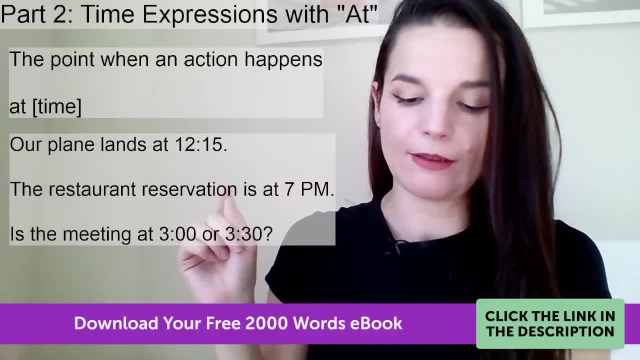 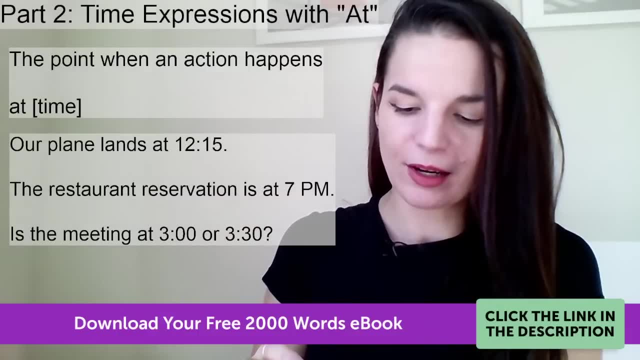 meeting Right M-E-E-T Right At 4 am. That's early Meeting at 4 am. Yeah, Juan says I always go to work at 6 am. Good, Augustin, the P-L-A-L. What does that mean? Plow? I'm not sure what that. 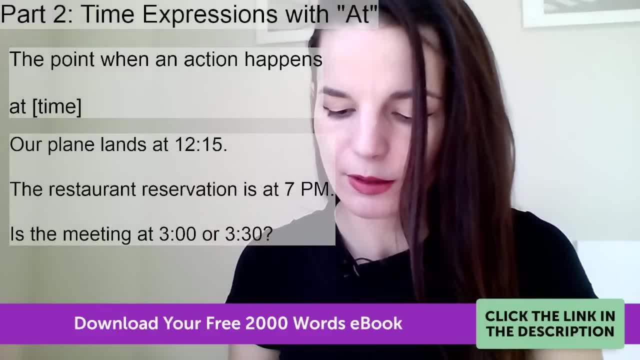 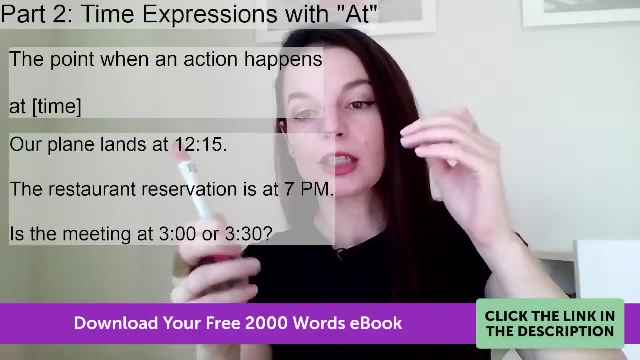 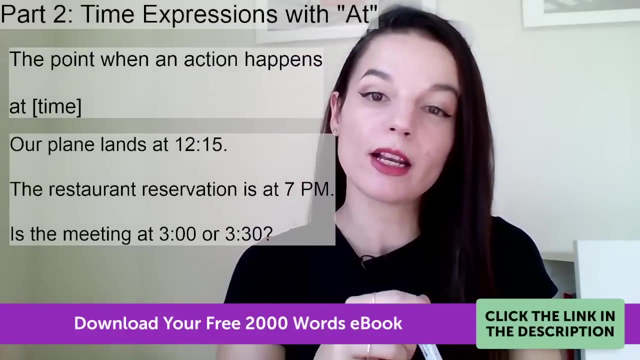 means, but maybe that's okay. I'm not sure what that means, but grammar is correct. I'm not sure what that is. Maybe the play will start at 4 pm, Not sure. Back to YouTube, Tolik. how do we use at on in for location? I have so many videos about this topic. Use your. 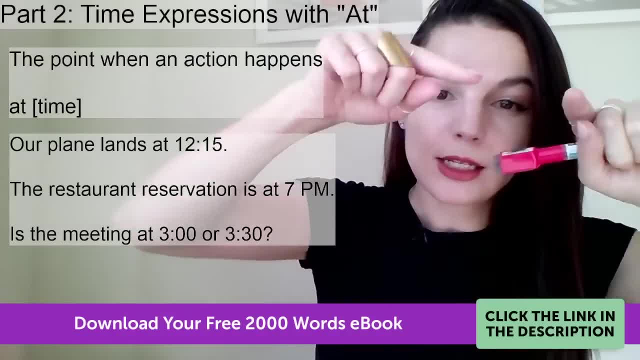 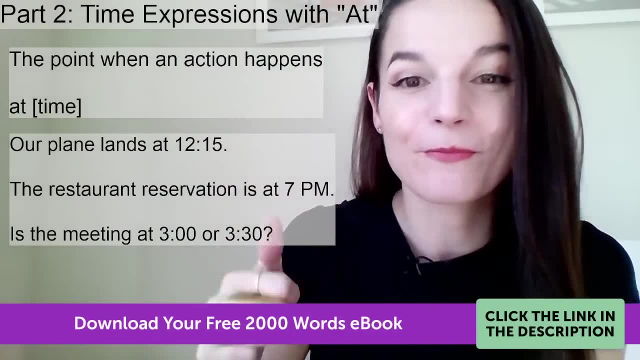 search skills on the YouTube channel. You are watching me on YouTube. Take your amazing eyeballs to the search bar at the top of the page and put at on in location. right there Got a bunch of videos. Okay, Let's see Other issues. 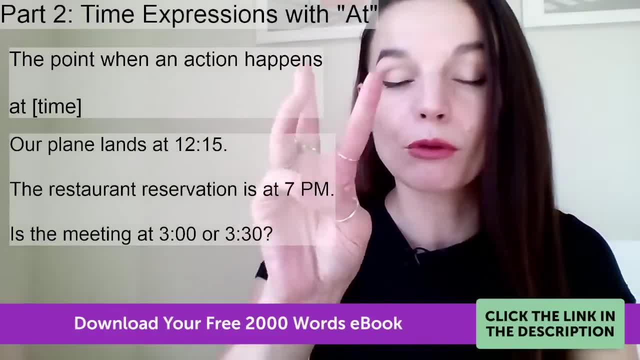 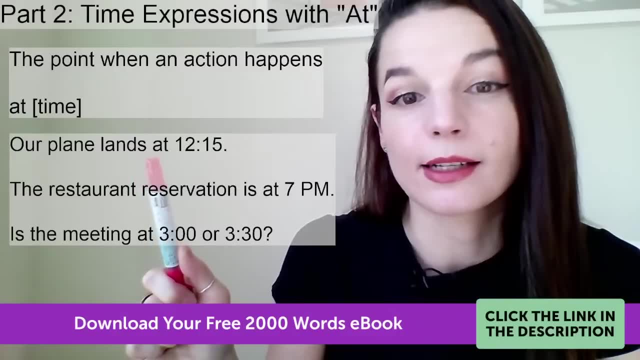 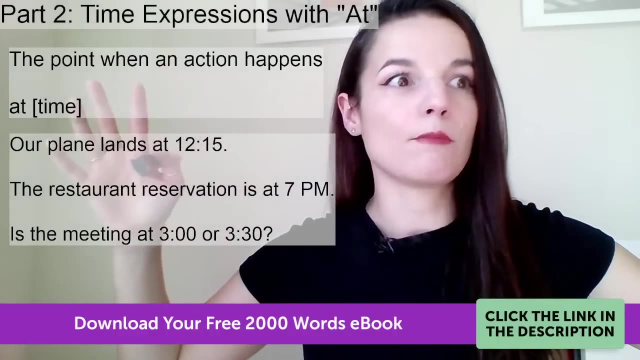 Okay, The one big one I see for many of you- I saw for three of you for sure, maybe more of you. don't forget your S for your present tense sentences. Yeah, The plane lands, Class starts, Practice ends, The movie begins. Right, Don't forget that little S there. I saw that a few. 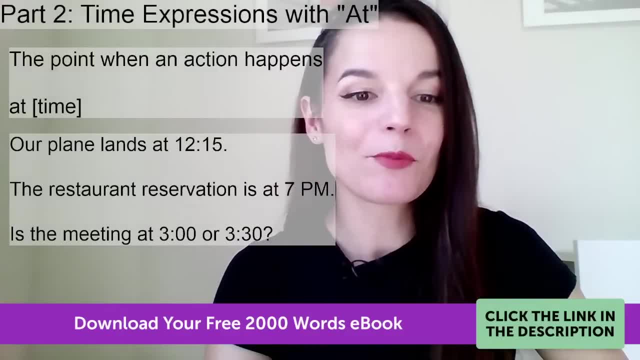 times. Okay, Let's finish there, because we have one more preposition to talk about. Meaning was good, Everybody got the meaning. Okay, Let's finish there, because we have one more preposition to talk about. Meaning was good, Everybody got the meaning. Okay, Let's finish there, because we have one more. 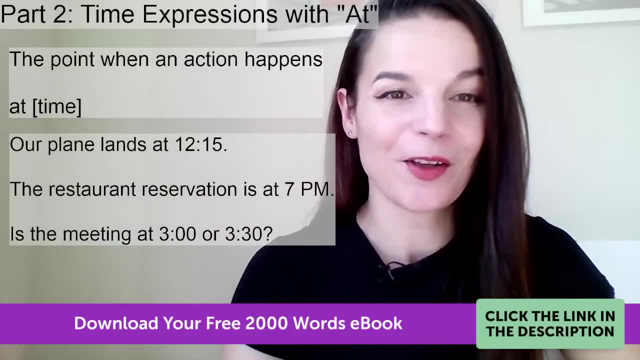 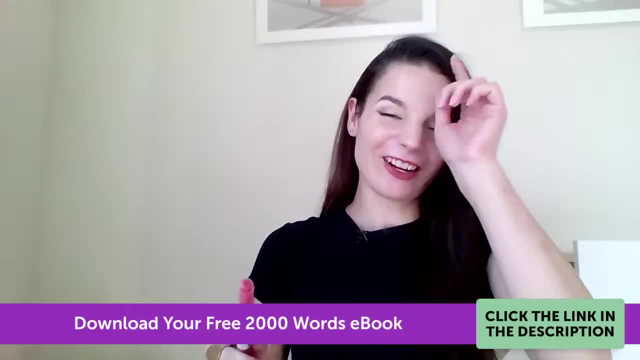 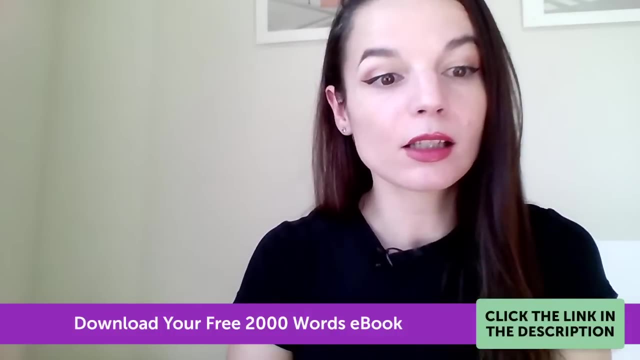 meaning good, but we need to review a different grammar point, I think. Okay, Alright, Let's take another very quick break. You can write your notes in your notebook while I do this. if you forgot or if you have not seen it, recently, our team has a new 2000 word e-book. This is a 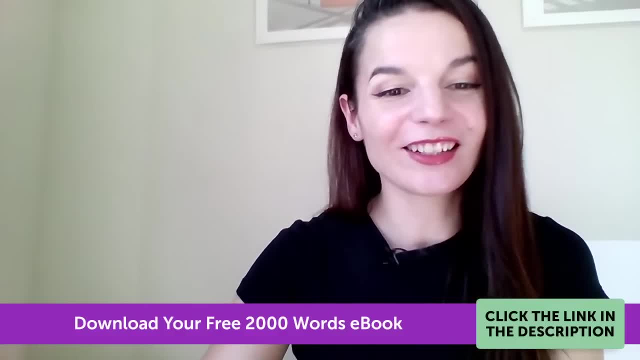 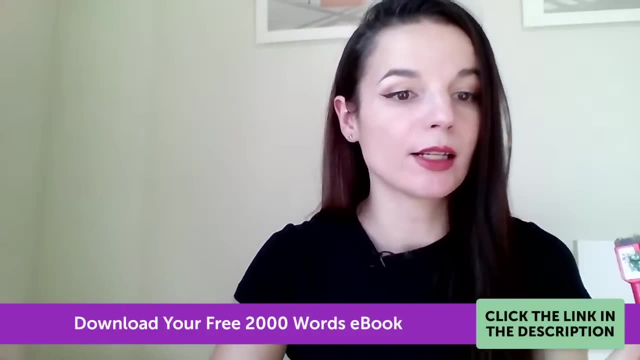 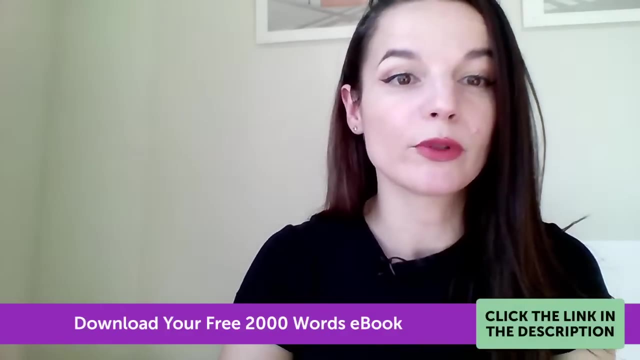 vocabulary study tool. So our team has created this e-book to make sure you study the most commonly used words first, So before you study something that not very often used, or to make sure, basically, you are most efficient in your studies. our team created this, so if you want to get this, you can get it for free. 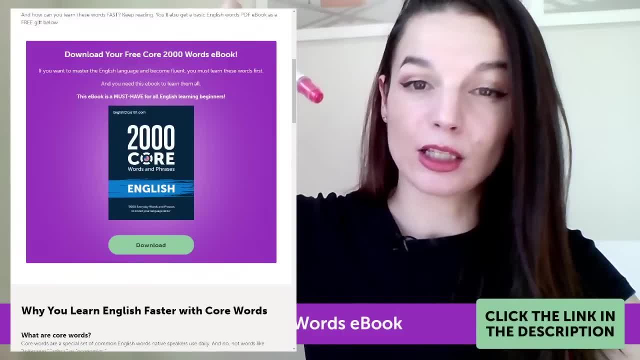 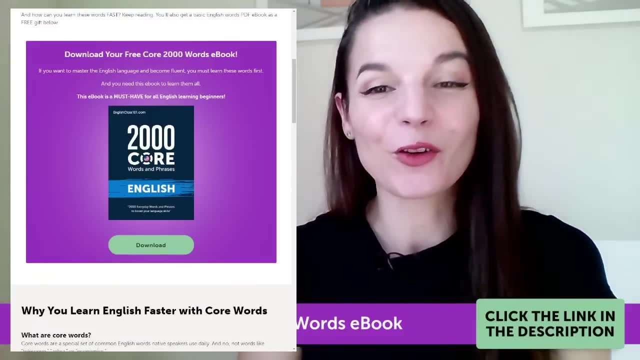 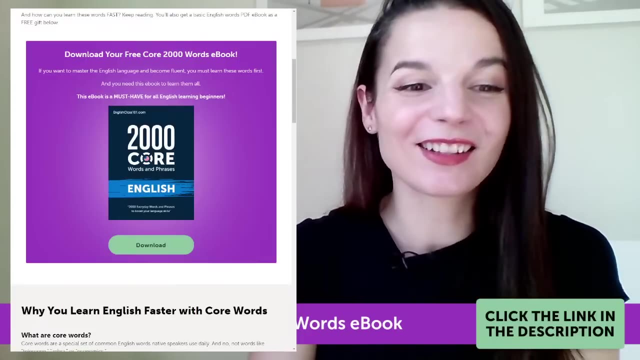 at EnglishClass101.com. the link is in the YouTube description or in the Facebook box, which is maybe here or maybe here, depending on how you're watching. on Facebook, you need your name and an email address and that's it. so, go crazy, get this. you can download this and study everything and get the most. 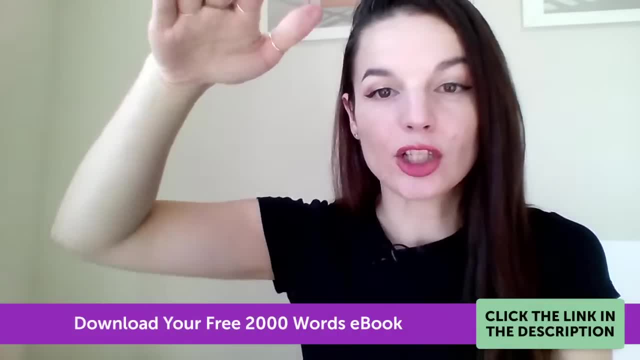 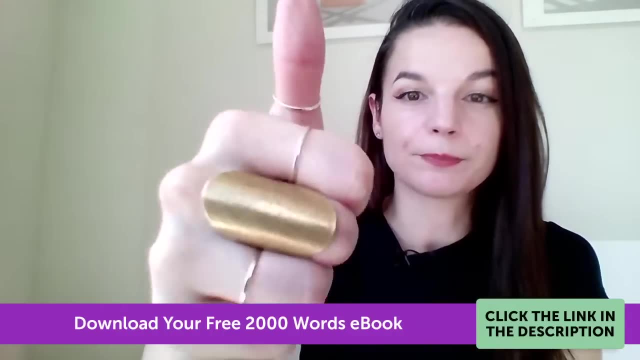 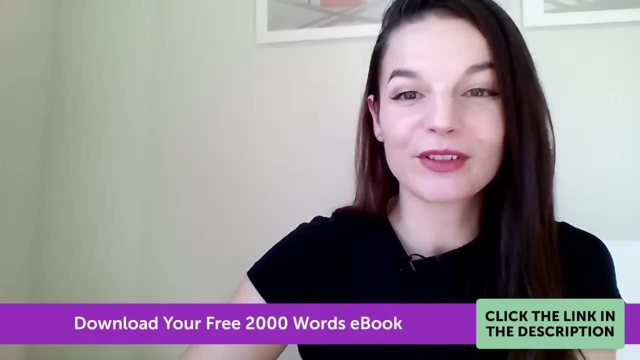 common words to help you get fluent faster. all right, let's go. so let's go to the last preposition today. if you have not, please make sure, hit the like button, yeah, and share this video so that others can find this life-changing preposition information never before seen on the internet. okay, let's go to. 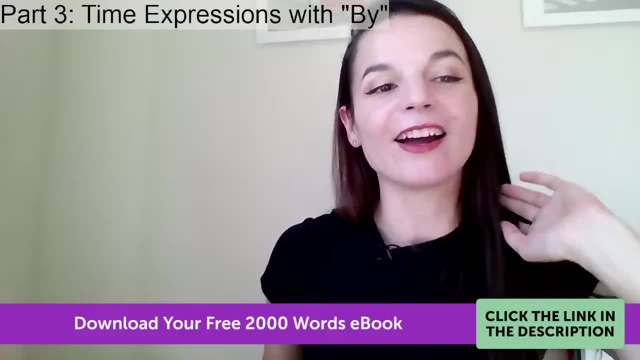 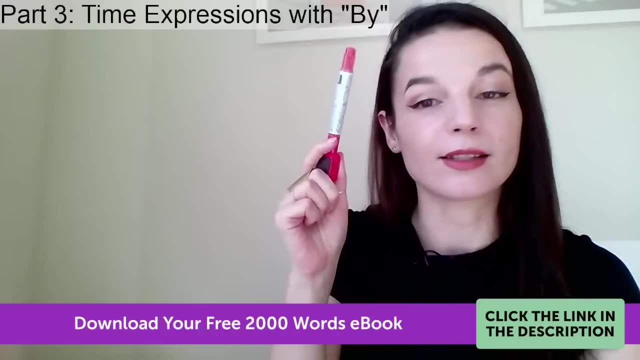 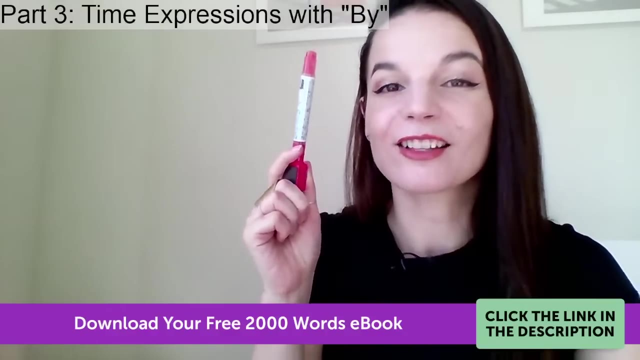 part three time expressions with by. okay, we're gonna talk about by. if you want to know about the difference between by and until, I am NOT going to talk about this today. I have a big lesson about the difference between by and until on the English class 101 YouTube channel, so please enjoy that after today's live. 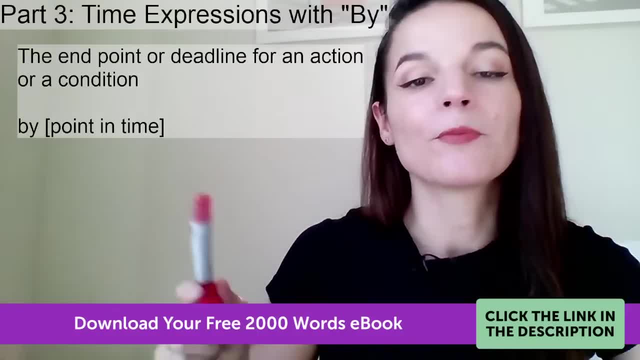 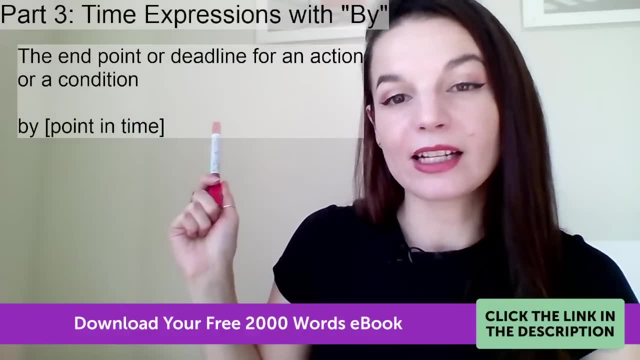 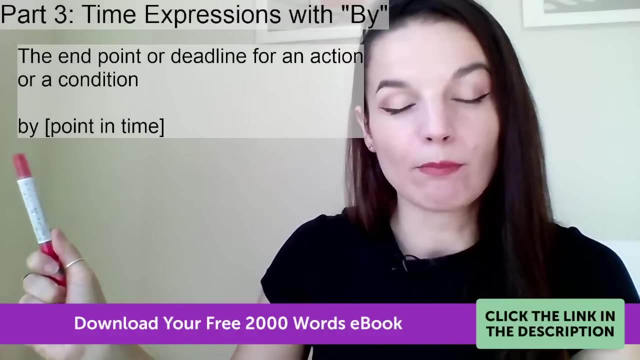 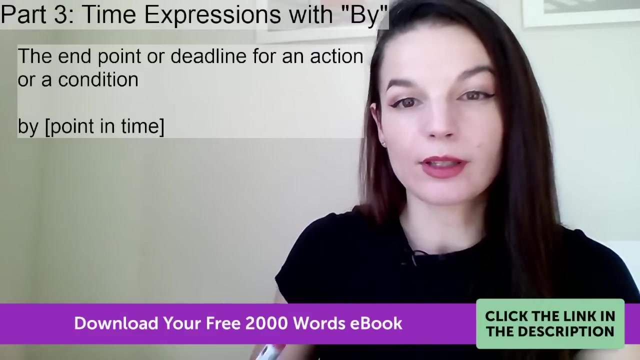 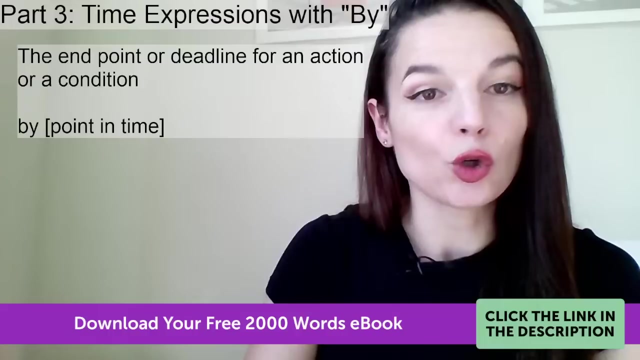 stream. let's talk about by only so we use by for the end point or deadline for of the question. okay. so the end point, the last point, them point in time, ok. so we're going to look at some examples and if we have time I will give you visual from sentences. you can send your examples of you very 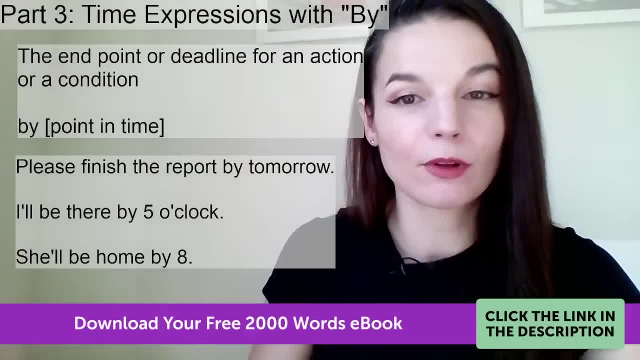 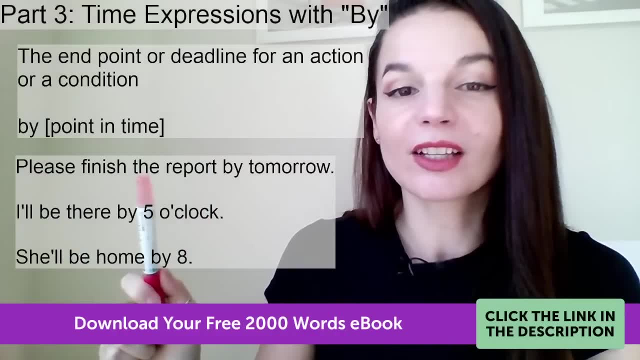 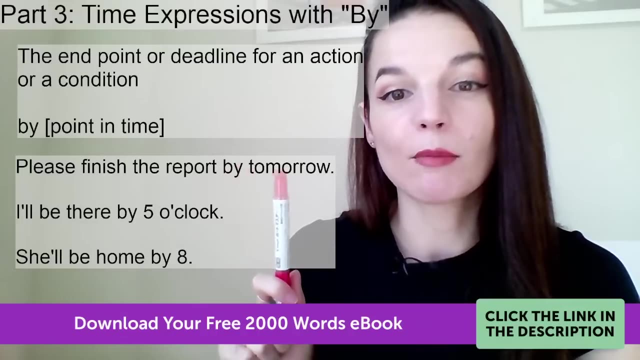 careful. this is the hardest one for today, k the one I see the most mistakes, mistakes. you watch the examples first. okay, First example: please finish the report by tomorrow. Please finish the report by tomorrow. This means tomorrow is the deadline for this. okay, So by tomorrow. 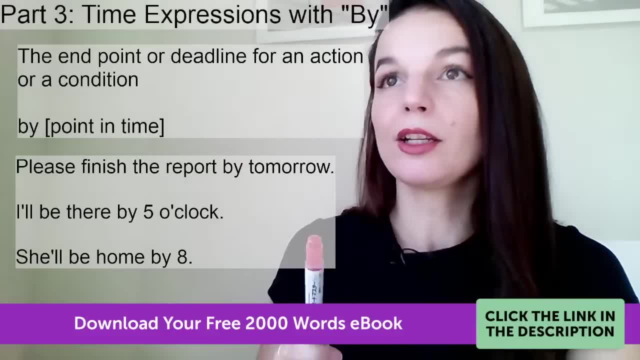 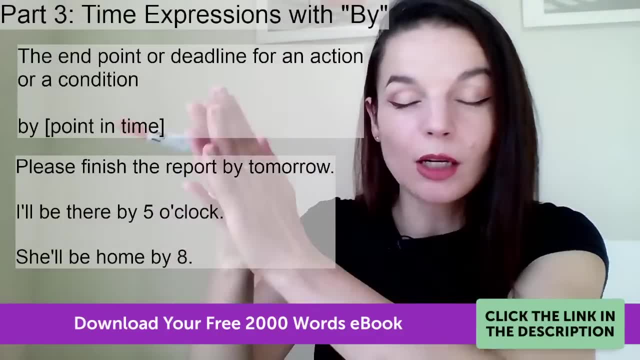 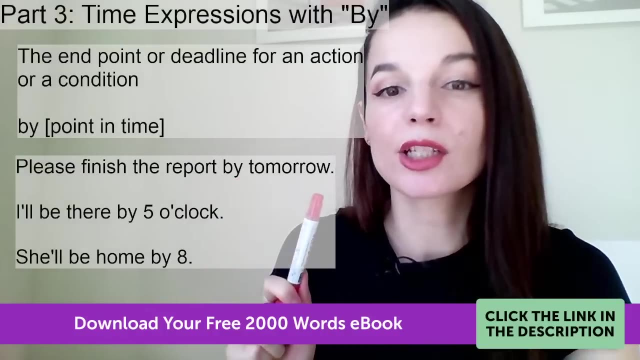 means if you finish the report tonight, great. If you finish the report in the morning, great, okay, By tomorrow. Tomorrow is the last point for the report, okay, So please finish the report by tomorrow. So tomorrow is our point in time. yeah, Tomorrow or two days from now. 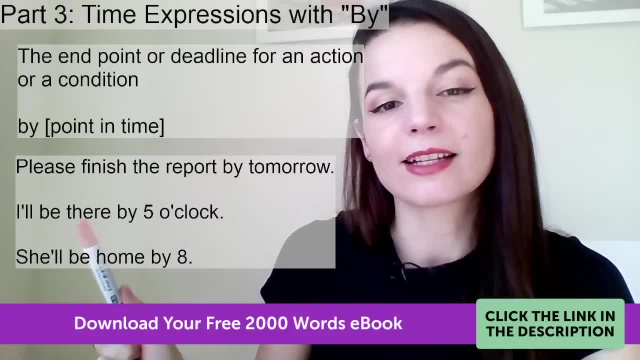 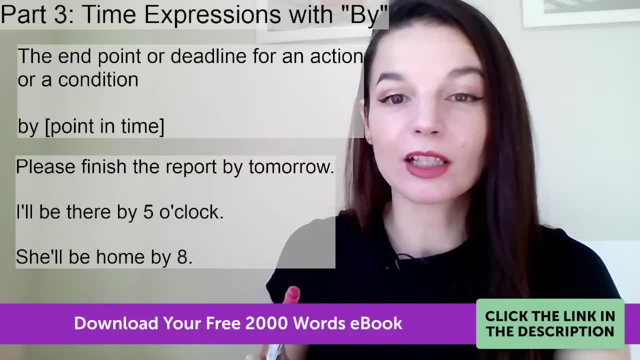 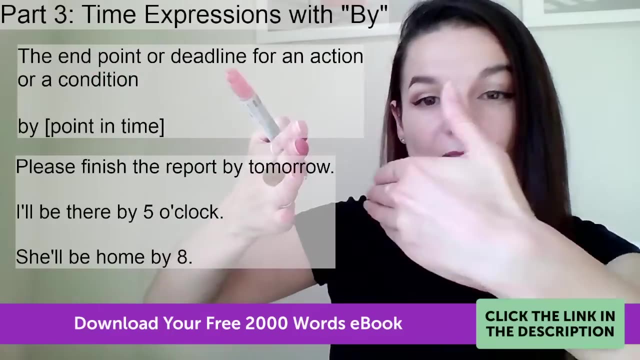 three days from now, right? Okay, let's look at the second example. I'll be there by five o'clock. I'll be there by five o'clock. This sentence means five o'clock is the last point, or the last point in time, the deadline for me to arrive, right? So maybe I will be there at 4.30.. 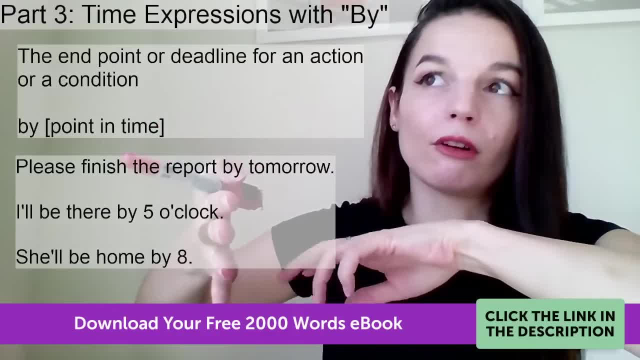 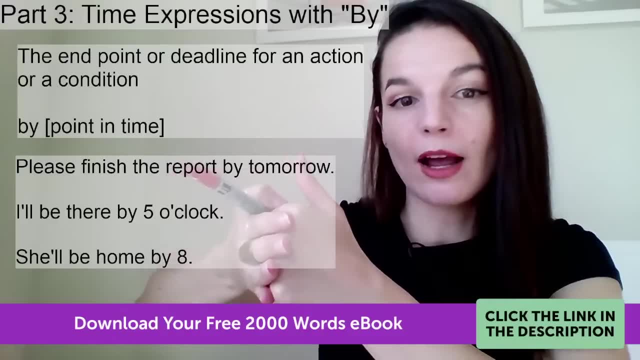 Maybe I'll be there at 4.40,, 4.45,, 4.50, right, But five o'clock is the deadline. That's the last point at which I will arrive, So you can use this if you are not sure, like I don't know. 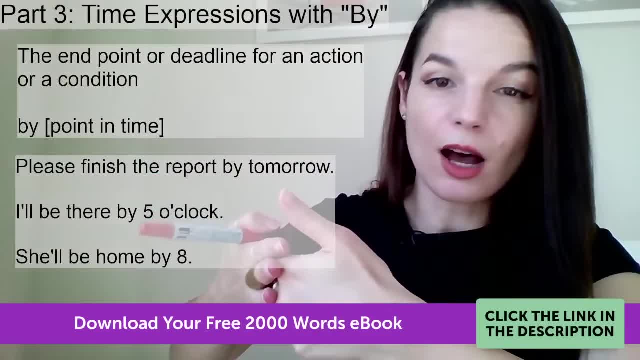 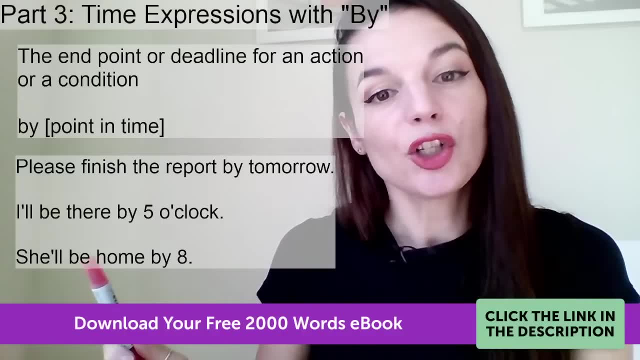 maybe 10 minutes, maybe 15 minutes. Okay, by five o'clock I'll be there. This is how we use this by Okay, last example, She'll be home by eight. She'll be home by eight. So again, this expresses: 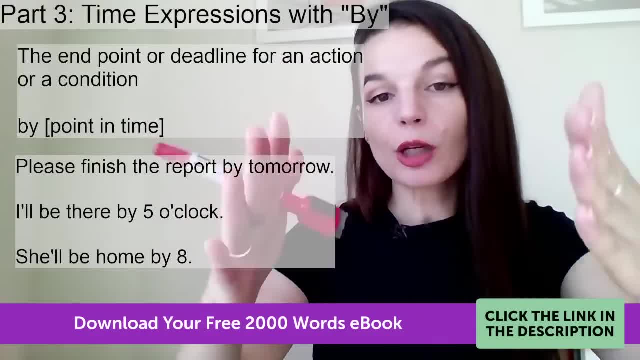 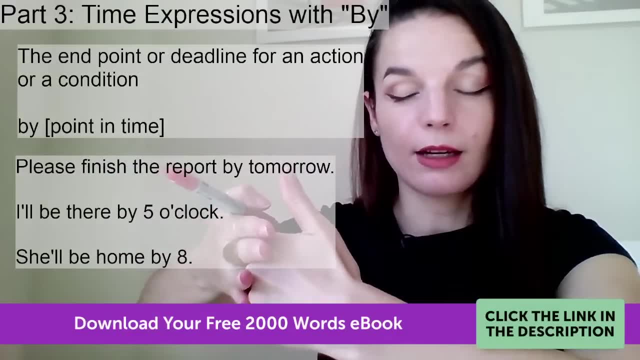 a deadline. Maybe now it's six. okay, She'll be home by eight. So again expresses the last point that we can expect, right? Or the last point for that action. okay, So before eight also okay. 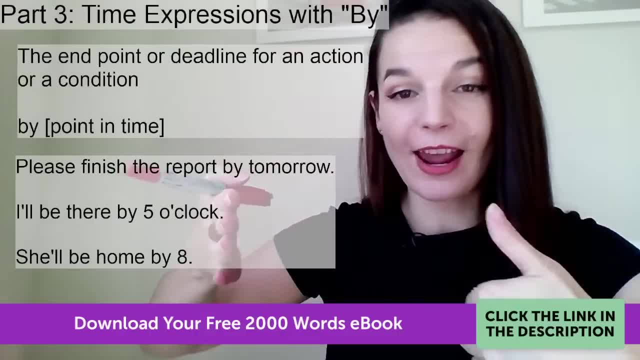 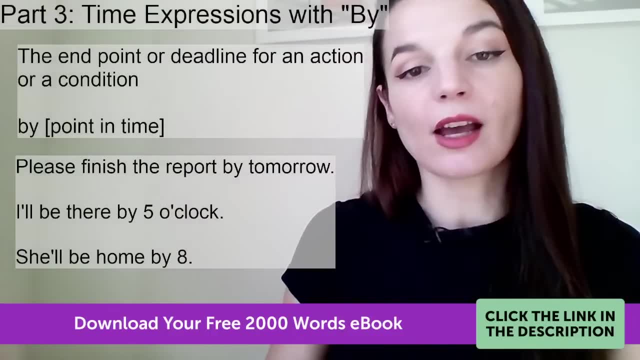 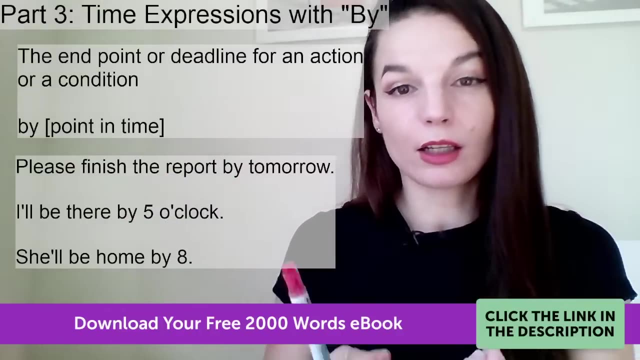 We can come before or she can come home before eight. Fine, Eight o'clock is the last point. So one other question sometimes learners have is like: can I say I'll be there at five o'clock or I'll be there at eight? Yes, those are grammatically. 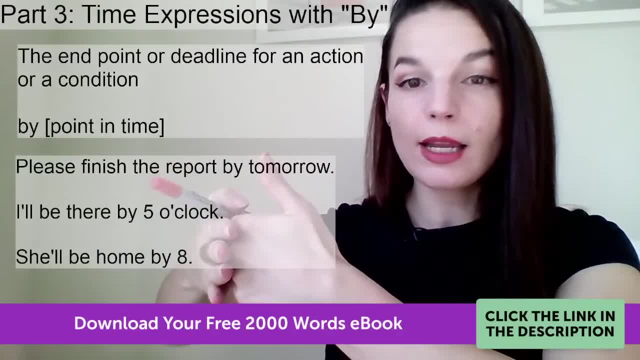 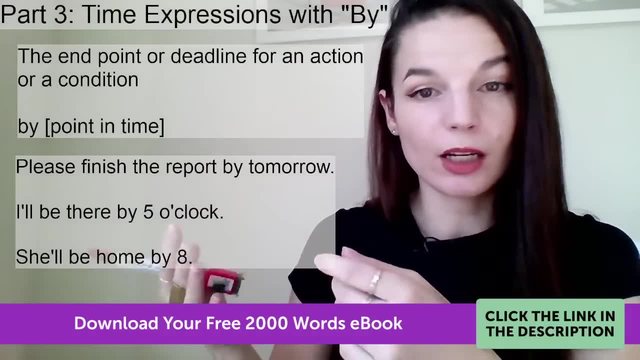 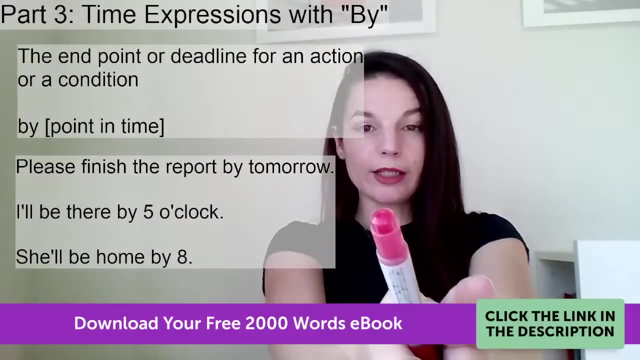 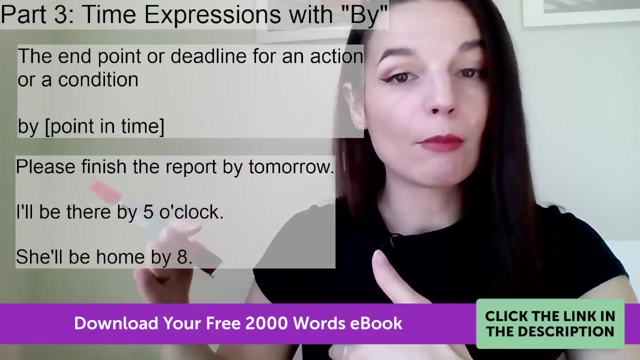 correct sentences. By communicates also before five o'clock or also before eight o'clock is possible, right? So by is really helpful to show a deadline for something. At marks the initial point, right. This is the time something will happen. By shows also the time before. 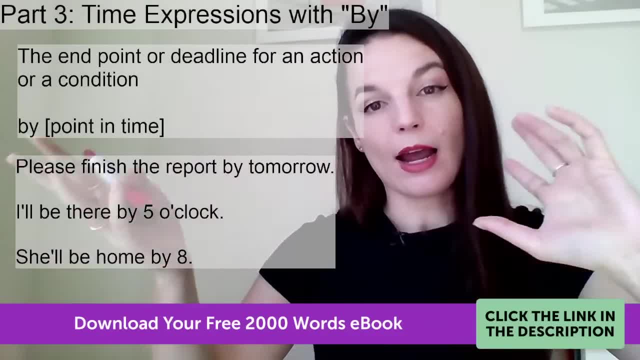 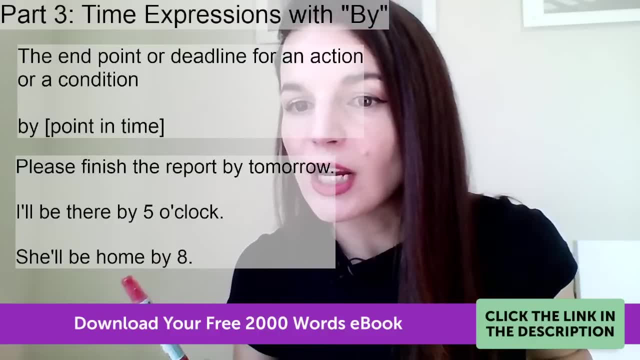 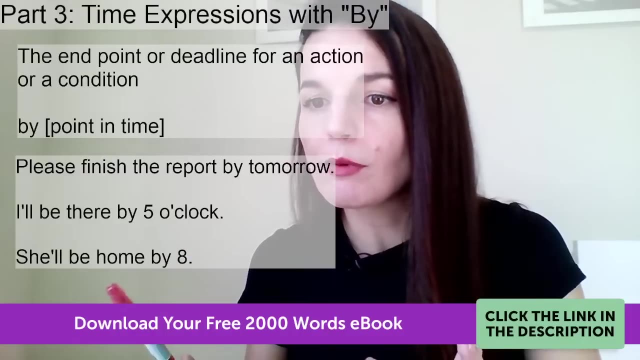 but not after. okay, This is how we use by and at differently. Okay, All right, I'm coming for your examples and your questions. I think I answered one already. Ninad wrote the video is going to be ready by today evening. We would today evening. you could just say tonight. 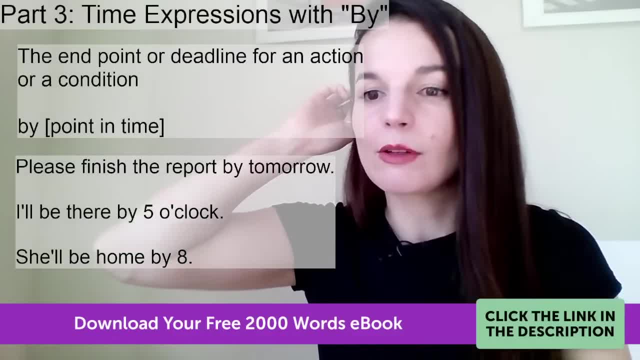 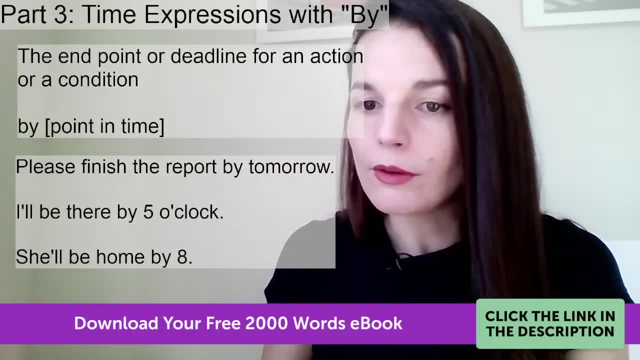 Okay, Tonight, right Tonight, That sounds more natural. The video is going to be ready by tonight. okay, Afghan wrote I will be in Kabul by 2 pm, Perfect, okay, Obaid wrote I will finish my. 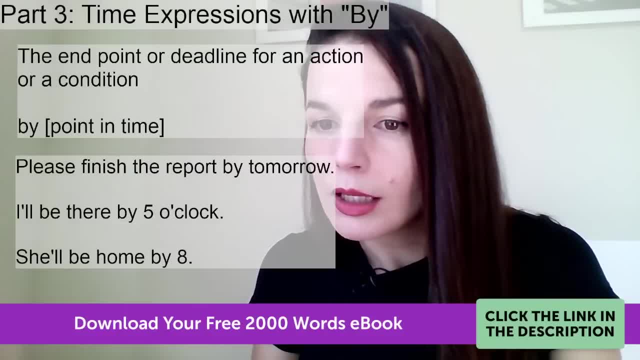 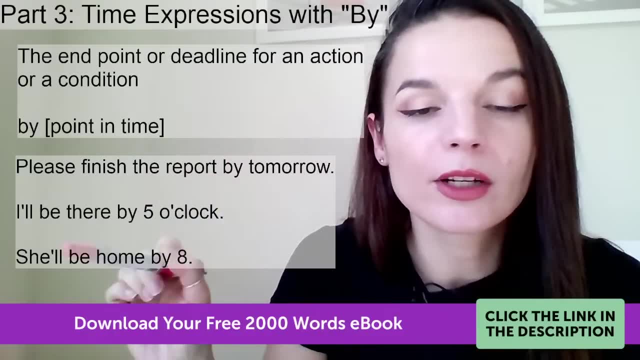 homework by tomorrow. Nice, Michaela, I'll, he, he, I'll, he'll, he'll, he'll. which one? All right, I'll maybe be in, don't forget. Oh, I don't have on this one. Be in the office by 10,. 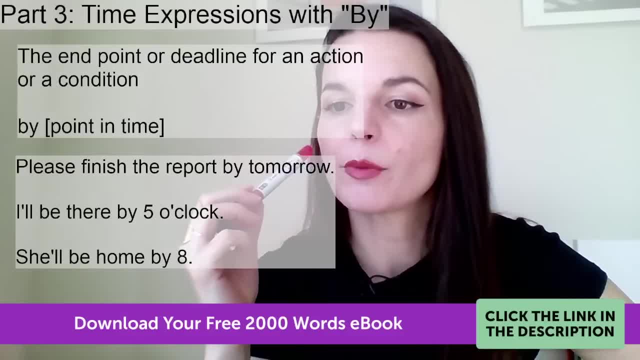 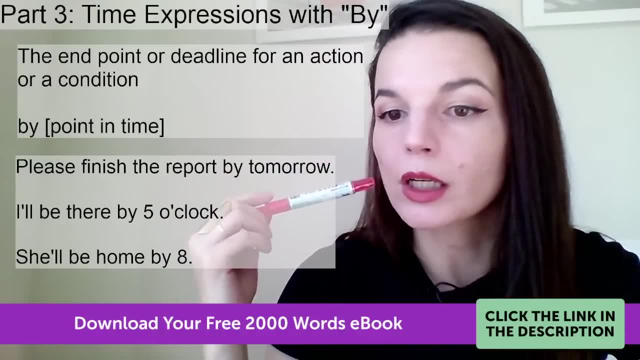 okay, And Jonathan wrote. can I say she'll be home By 8.30 am. Yes, that sounds fine to me, Max, the work, it is going to be finished by tomorrow. Just say the work is going to be finished. yeah, You don't need to say the work, it is right You. 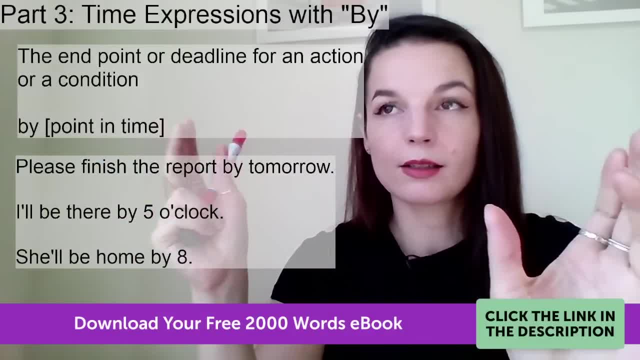 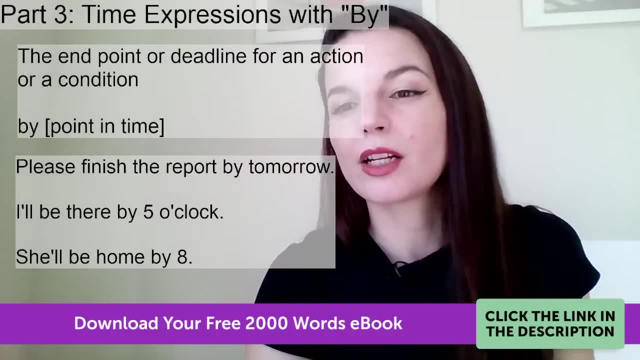 already have your subject, the work, right? So if you say the work, it is, it's like the work and it are the same thing, right? So get rid of it. yeah, The work is going to be finished by tomorrow. 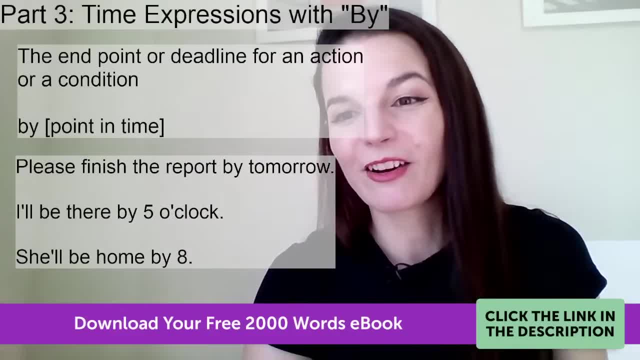 And Gustavo wrote: I have to find a birthday present by November. Swap those birthday present by November, So get rid of it. yeah, The work is going to be finished by tomorrow. birthday present by November. I can't read your name, I don't read the script, but I will buy a. 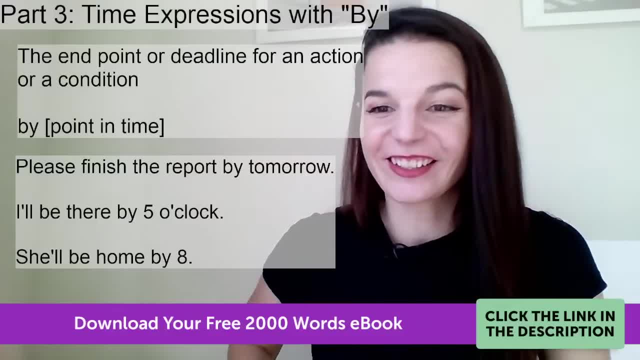 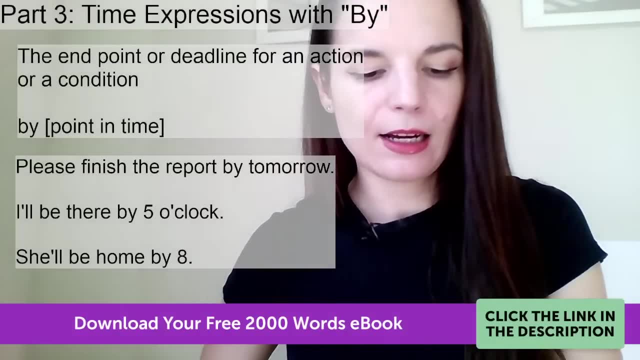 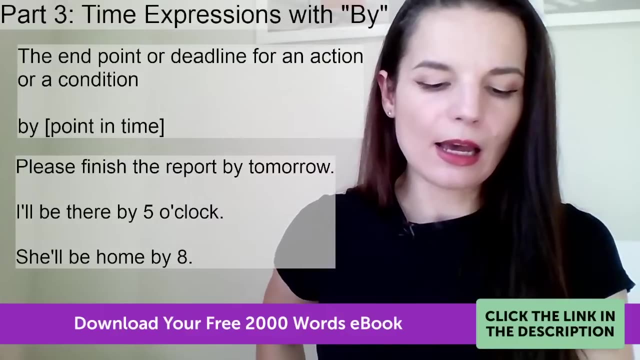 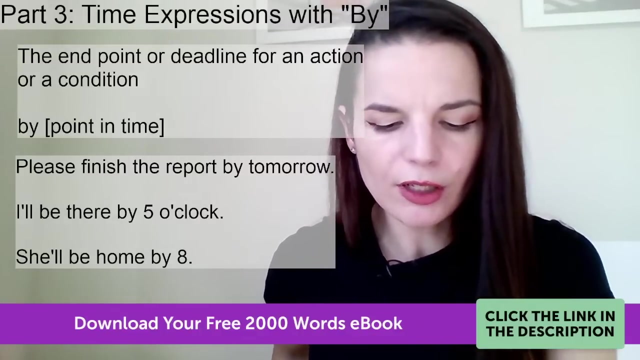 Mercedes by the summer. Okay, good luck. Good luck to you, Facebook. do you have some examples? Let's see? Rosa said: please finish the homework by tomorrow, okay. And July wrote: they will be at the playground by evening, okay. Ellie wrote: I will finish the. 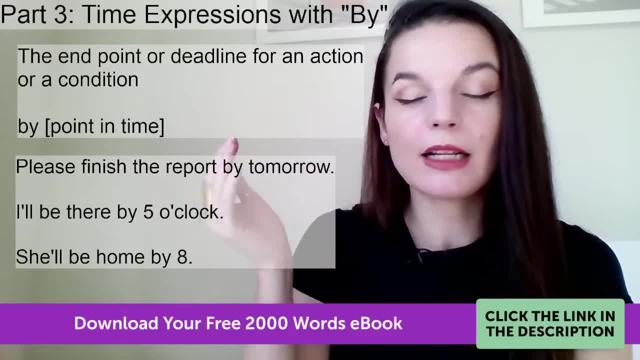 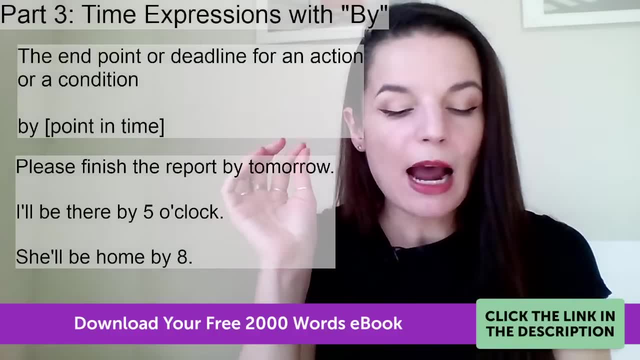 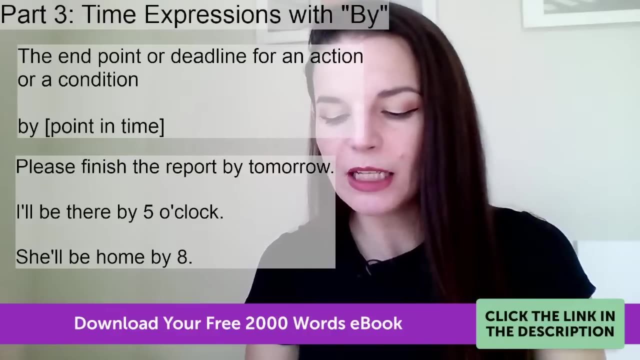 work by 15 minutes, So I'll finish the work in 15 minutes. If you want to talk about like something that you're imagining to do, like I will be finished with the work within 15 minutes or I will finish the work in 15 minutes, we would use in for that one. yeah, So that one we would. 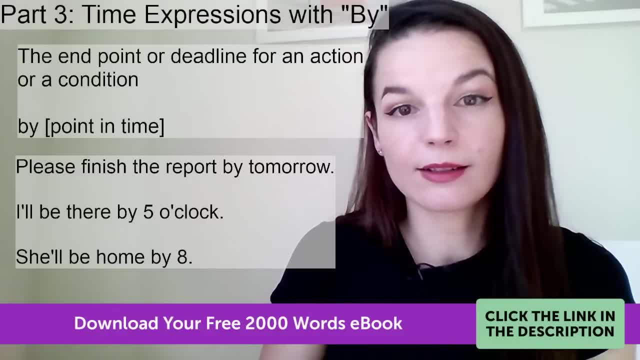 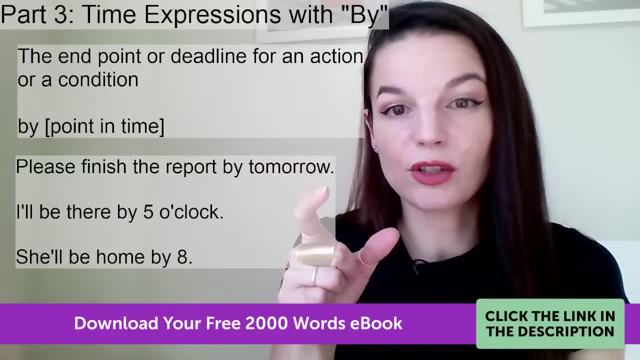 use in for I'll finish the work in 15 minutes, yeah, Okay. So I would say for those kinds of short periods of time, Like it sounds a little more natural to use that in to show I might do it before 15 minutes. 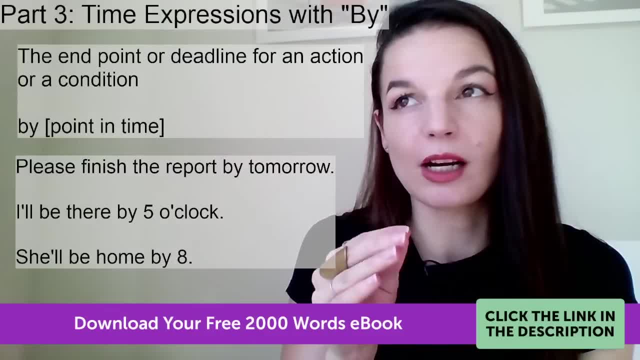 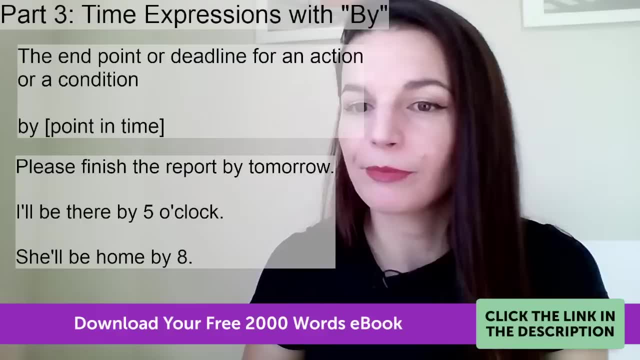 but because it's such a short period of time, I think it's more natural to use that I will finish it in, or you could say within 15 minutes. That's a good choice. Okay, And all right, I have to. 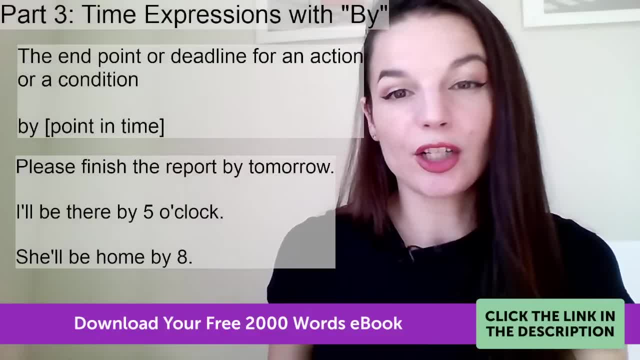 finish. Oh my gosh, time went so fast. So this is a quick introduction to using by and at and in for today, But, as I mentioned, I have a lot of time. I have a lot of time. I have a lot of time I have. 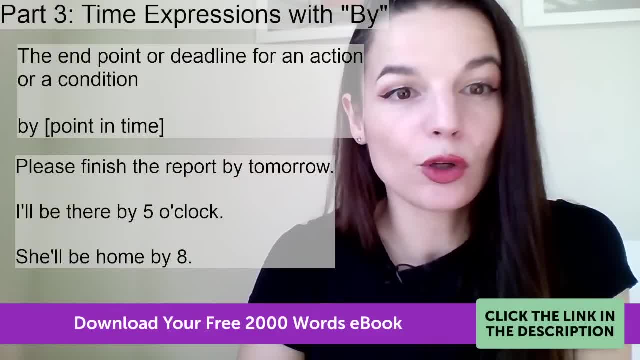 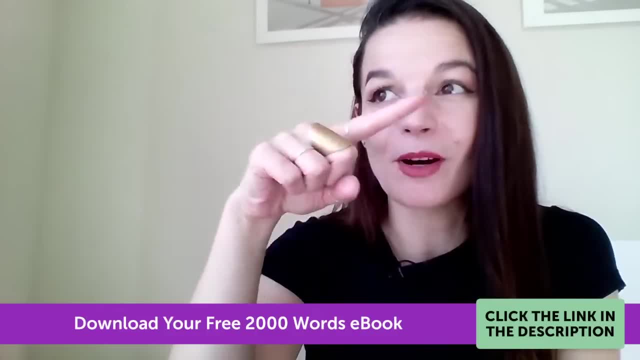 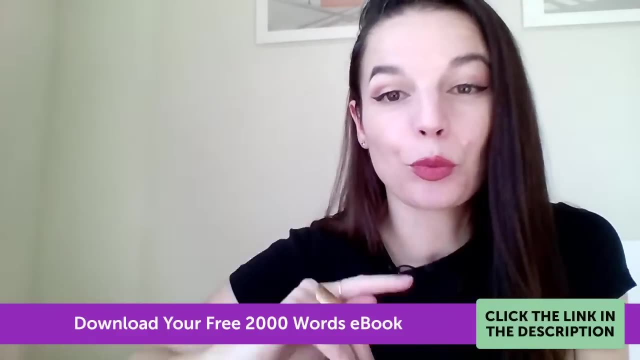 a lot of videos on these topics, So you can use the search bar. If you're watching on YouTube there's a search bar that you can type by at in You can type preposition. You can use that search bar to find lots of my videos from the last many, many years to practice these points in more. 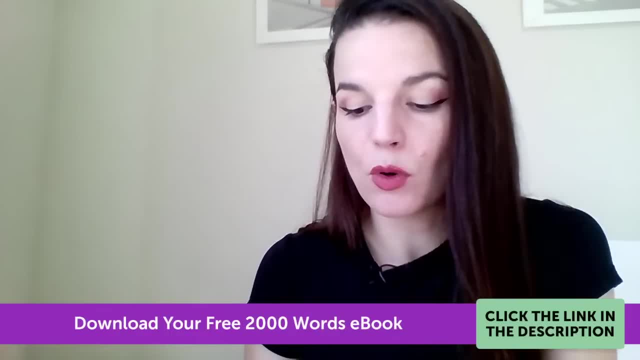 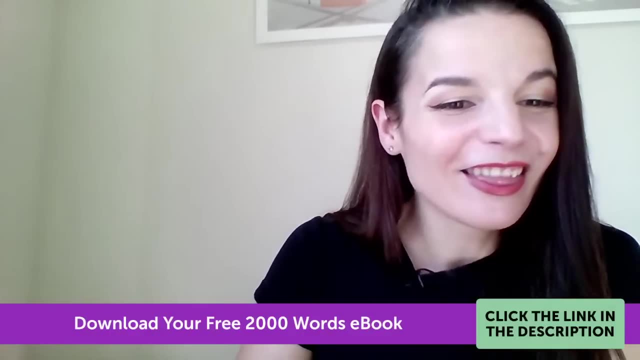 detail, So I recommend you do that. if you have some more questions, Okay, But I have to finish for today's time, So let's finish up. Let's see Next week's lesson information. Where'd you go? Okay, here it is, So I'll be back. 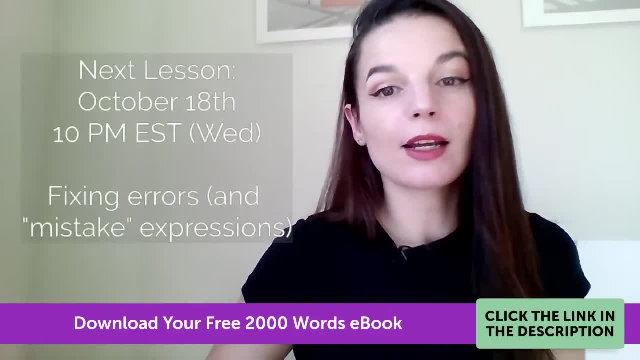 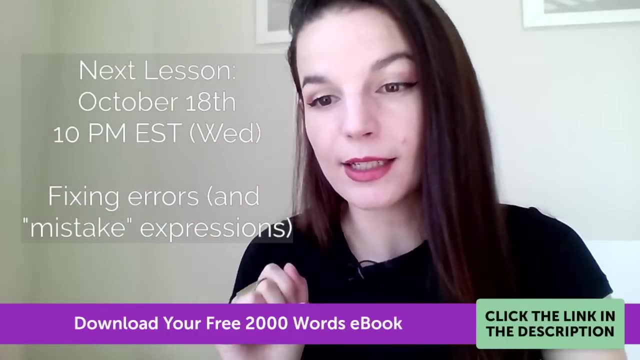 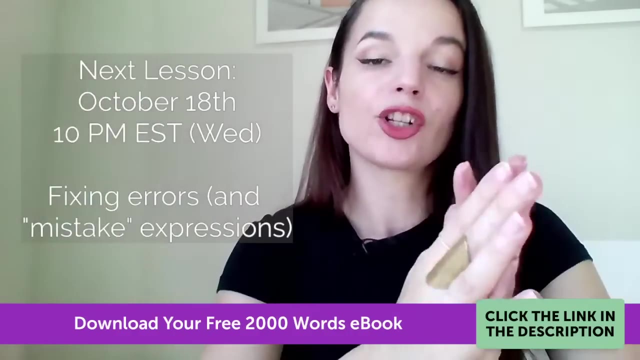 next week. Of course, we are going to talk about a different topic next week, though, So please join me next week, Wednesday, October 18th, at 10 pm Eastern Standard Time. That is New York City time. If you don't know your local time, please Google it or set a notification on YouTube or on Facebook. 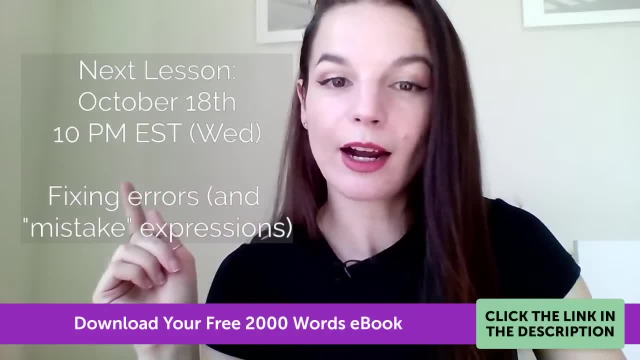 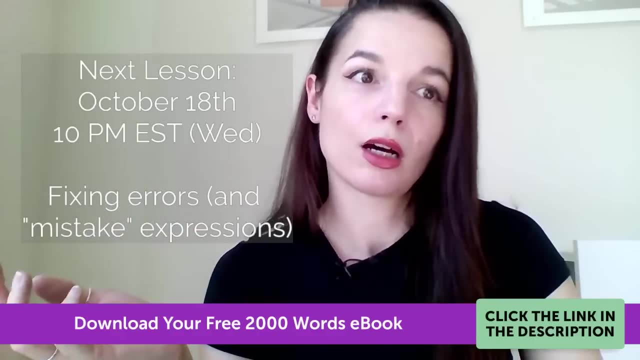 so you don't miss the session Next week. I'm going to talk about fixing errors and mistake expressions. So like, how do you say, like- maybe some of you know- like oops or uh-oh or those kinds of things, but just more of that. So we're going to talk about how to 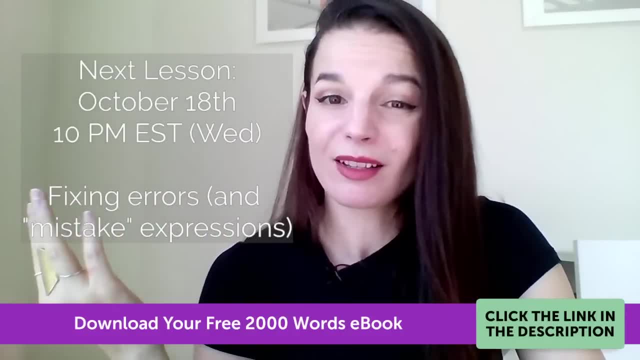 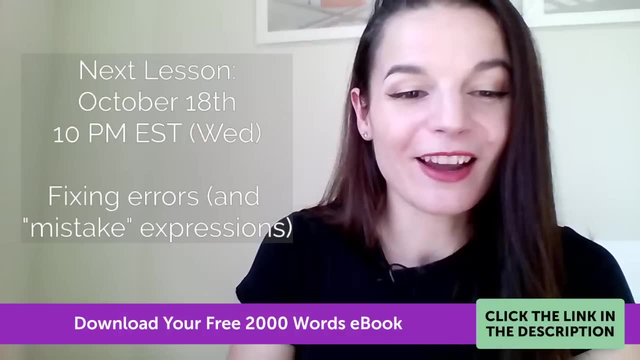 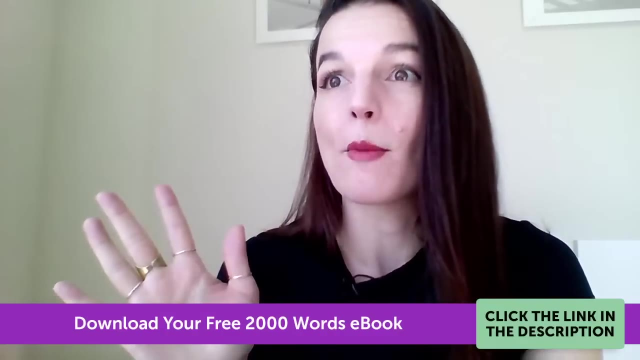 fix these kinds of things and express when we have made a mistake, because it's important, right? I hate to make mistakes, but it happens to the best of us, So please join me again next week for that. Again, if you want more preposition practice, go crazy on my past videos I have so. 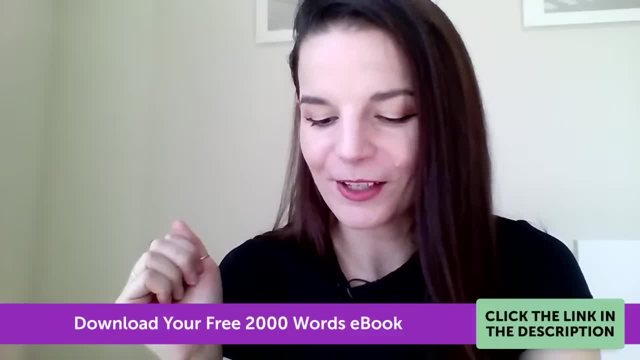 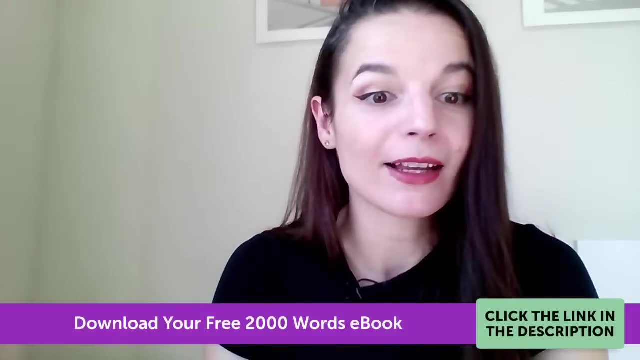 many, And that's it. That's all for me. Don't forget your free 2,000 words ebook that our team has made recently. This is- yeah, this is fresh. This is fresh off the fresh out of the oven, So please. 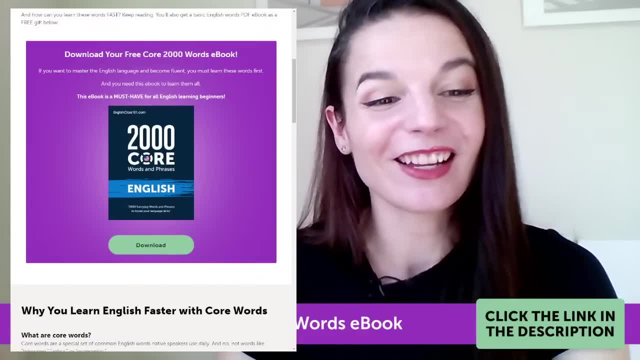 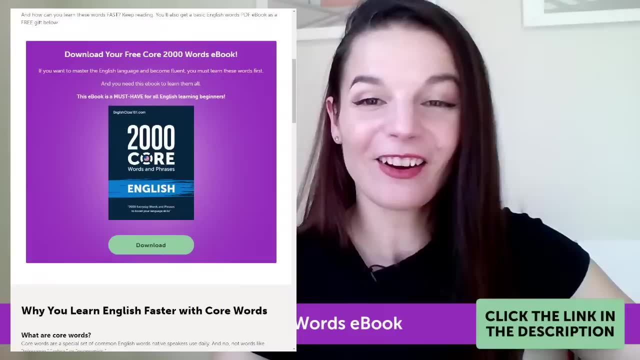 go and enjoy this. This is a great vocabulary study tool So you can make sure you study the most important words first right, Use your time in the best way. All right, That's it for me. You can come and find me on Instagram. I'll see you next week. Bye. 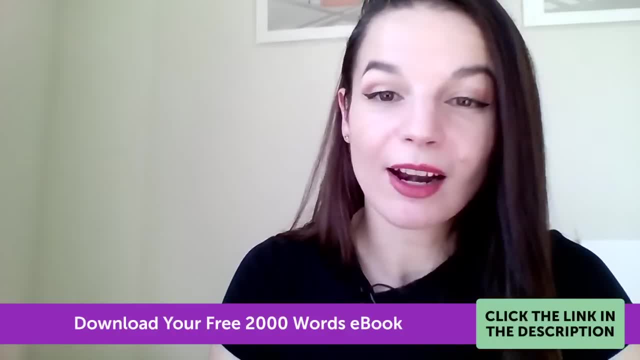 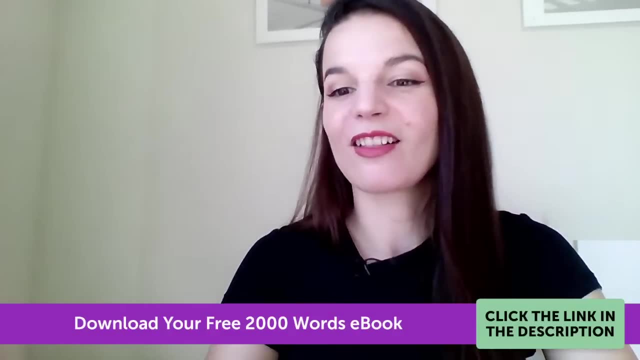 Instagram after this And you can come and find our team at English class 101.. And I hope you have a great day and a great evening, a great weekend, wherever you are in the world, And I will see you.